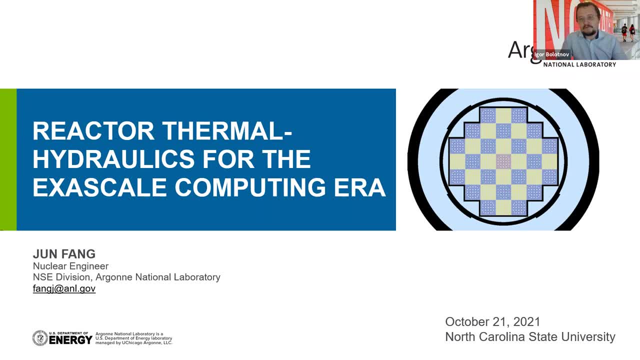 And I'm looking forward to hear what's going on in his research career nowadays. And please welcome our speaker, Dr Jin Fang, By the way. quick thing, Yeah. So if you do have questions, please do post them in the chat. 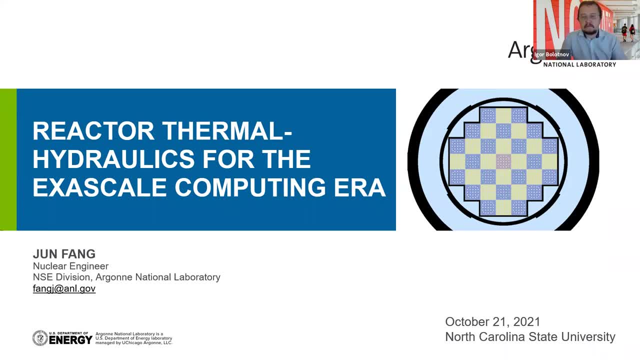 And then In the end we will try to. I think Professor Shannon will help us out with the audience questions and then with the chat questions as well. All right, Thank you. Please go ahead, Jin. OK, All right, Thank you for the introduction. 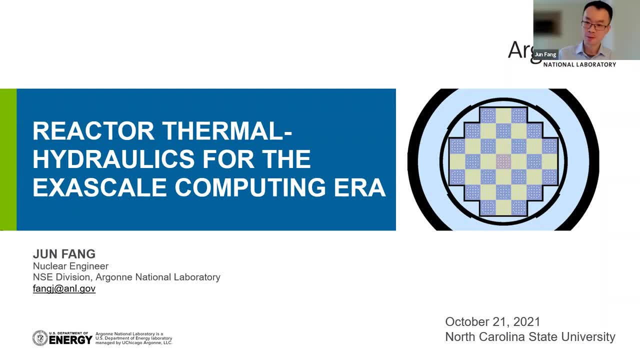 I'm glad to be here. So I've been working at Argonne for more than four years since I graduated from NC State. I still remember the days coming to Burlington for the seminars. Let me guess today You probably only have some soda and cookies. 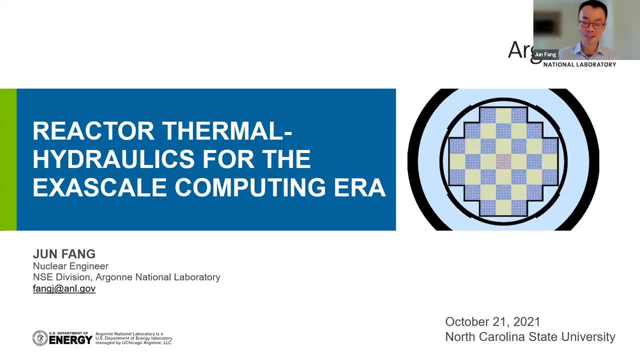 I remember back then, whenever there's a big guy giving the seminar talk, there'll be a lot of fruit and even pizza or pasta. I still remember those days So well. anyways, the topic of my talk today is reactor soma hydraulics for the exascale computing era. 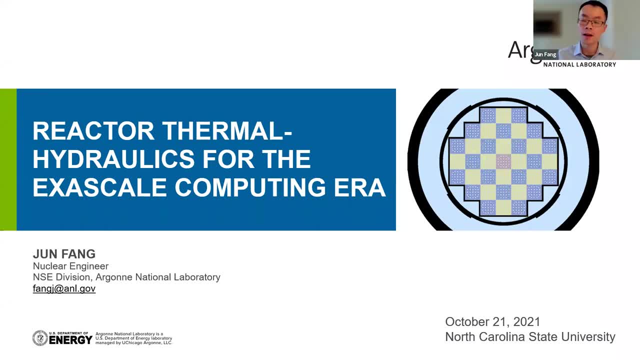 And here you will see, as nuclear engineers, how we prepare ourselves for the coming of exascale computing, And the research I'm going to present is a team work involving multiple national labs and universities and led by Argonne and Oak Ridge. So let's get started. 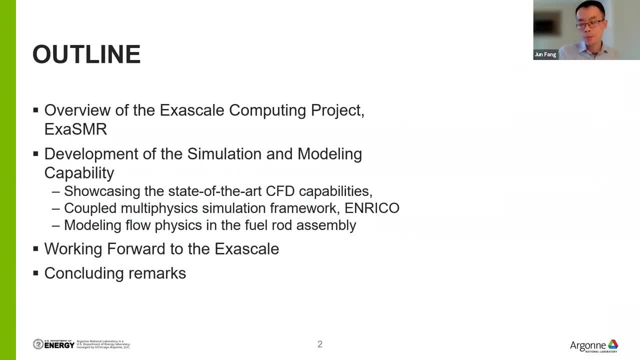 Here's an outline. The work here is funded by the DOE exascale computing project, So I will first give an overview about the project background and its mission. that is to develop the multi physics simulation capability for nuclear reactor system. Specifically, we're targeting the small modular reactor design by new scale. 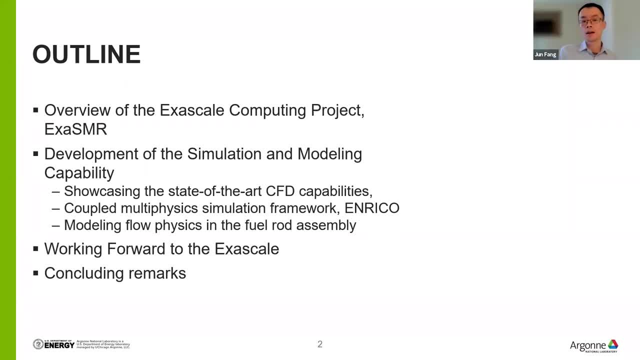 And around this mission. in the second part, I'm going to introduce the development regarding the simulation and modeling capabilities, which includes some highlights about our state of our safety capabilities. So we're going to talk about some highlights about our state of our safety capabilities. 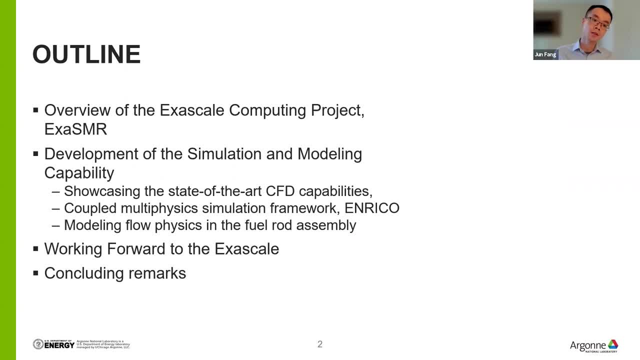 So we're going to talk about some highlights about our state of our safety capabilities. So we're going to talk about some highlights about our state of our safety capabilities And I'll also briefly talk about the coupling framework, which is Enrico, which brings together the eutronics and CFD. 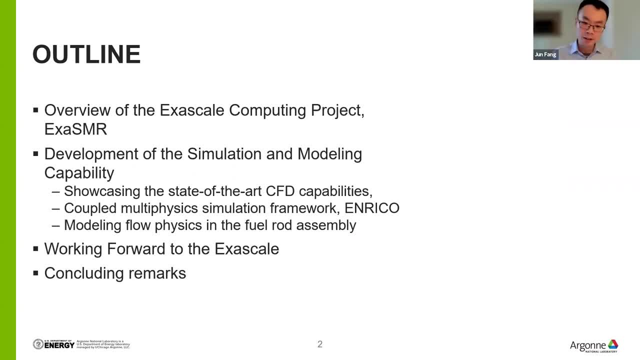 So in the real nuclear reactor core there are a lot of detailed geometric structures. even with the exascale supercomputer We won't be able to resolve all these geometric details, So instead we will have to develop some. So instead we will have to develop some. 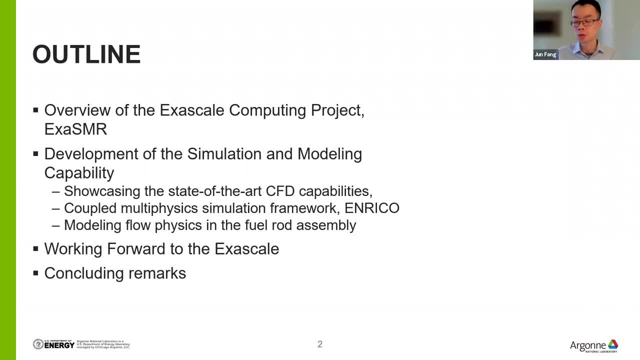 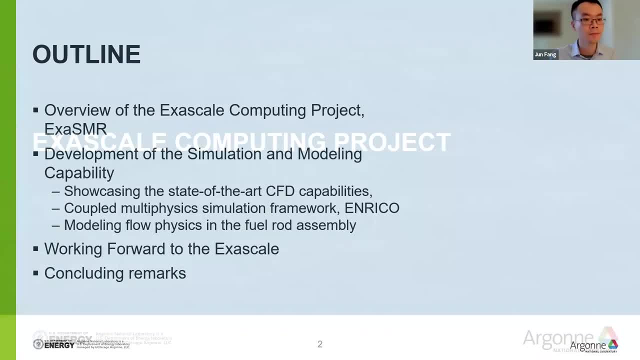 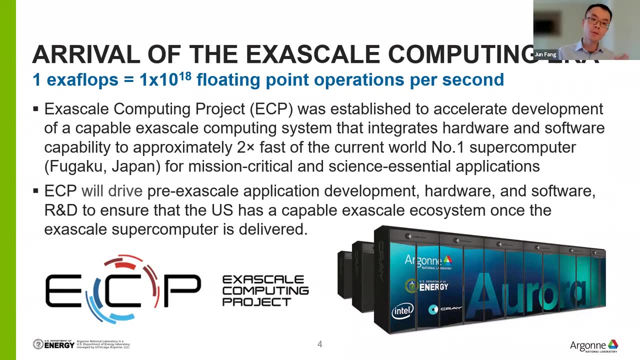 And then I will end the talk with some close concluding remarks. So what is exascale? An exascale supercomputer means it can perform 1 billion billion floating point operations per second. So that is 10 to the power of 18.. 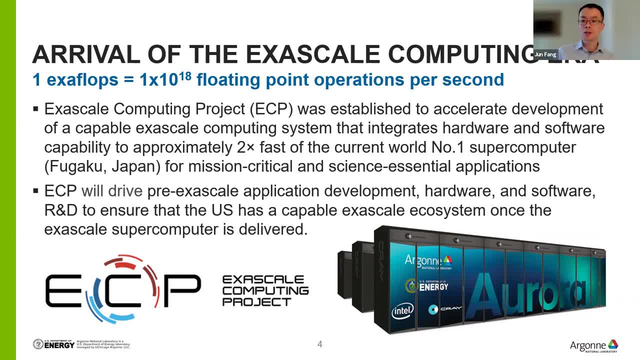 And to put it into context, the current world number one supercomputer is this Fukaku supercomputer in Japan, which has a peak performance, about 500 petaflops, And the current fastest supercomputer in the universe. The first one in the US is the Summit supercomputer at Oak Ridge, which has about 200 petaflops. 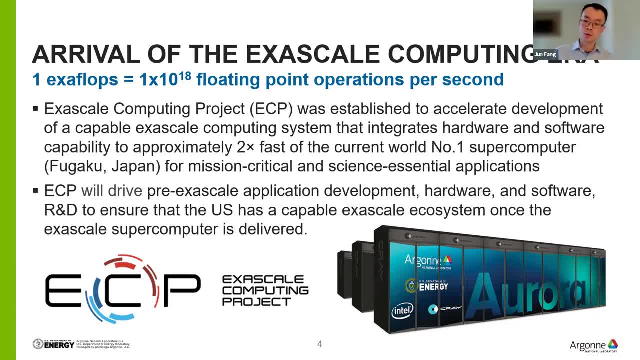 And one exaflops is 1,000 petaflops, And we want to lead the game, so we are building exascale supercomputers. One of such examples is Aurora being built at ARGA, which has at least one exaflops performance. 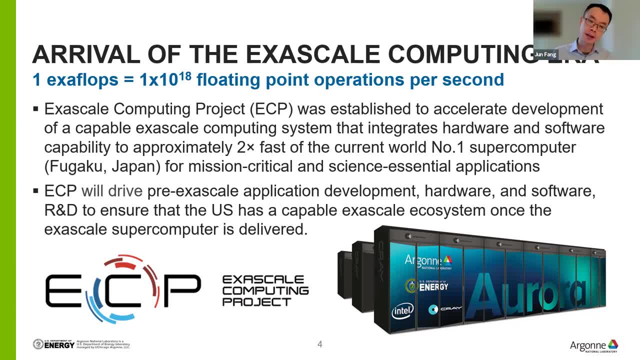 So, as a response to this, I am going to give you the example of Porf John. In response to the arriving of this exascale computing era, the ECP was established to accelerate the development of a capable exascale computing system that integrates both the hardware and software for the mission-critical and science-essential applications. 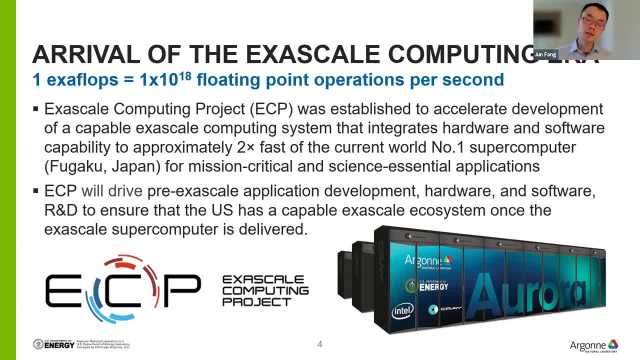 So I also want to clarify here: the ECP will not be responsible to build these supercomputers. Instead, it will drive the pre-exascale application development and make sure the US has a capable exascale ecosystem once the new supercomputer is delivered. 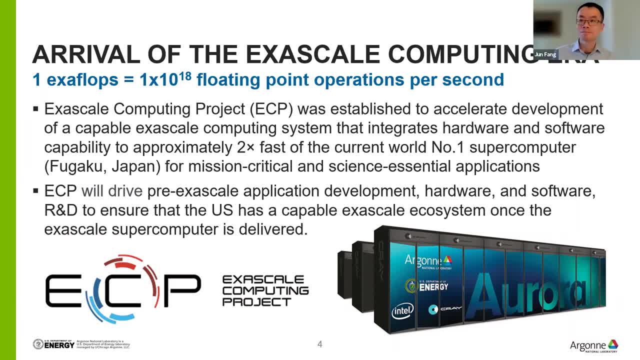 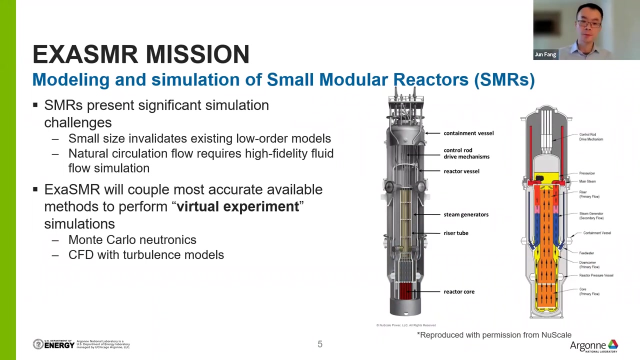 So you may ask what the exascale supercomputer can do. So, from the traditional, you know- weather forecast and predicting the climate change, to assimilating the galaxies and even mapping the neurons in the human brain. And among these ECP priorities, there's one specific to nuclear engineering, that is, to develop the simulation- multi-physics simulation capability for the new reactor system. 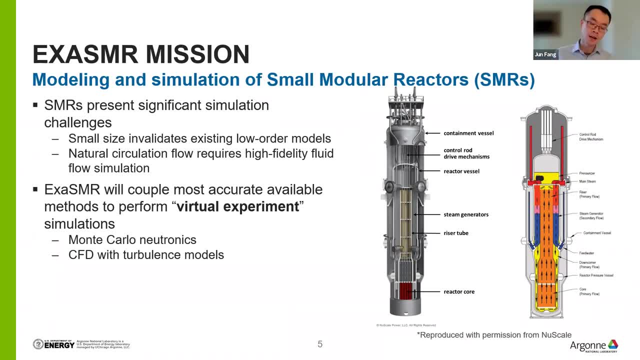 And, as I mentioned earlier that our target is the new system And, as I mentioned earlier that our target is the new system And, as I mentioned earlier that our target is the new system. So we have a very scale small modular reactor design. 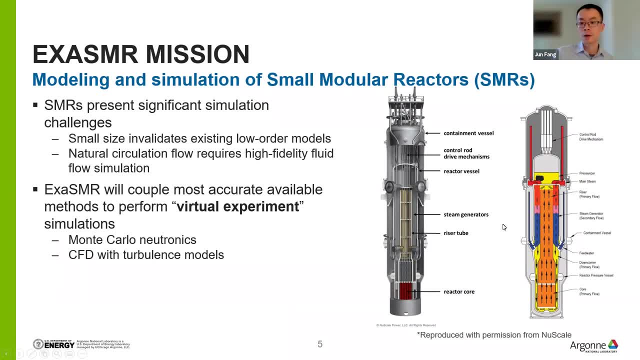 On the right hand side you can see a sketch about the SMR system. On the bottom we have the reactor core And then in the middle we have the steam generator And then on the top there's some control devices. 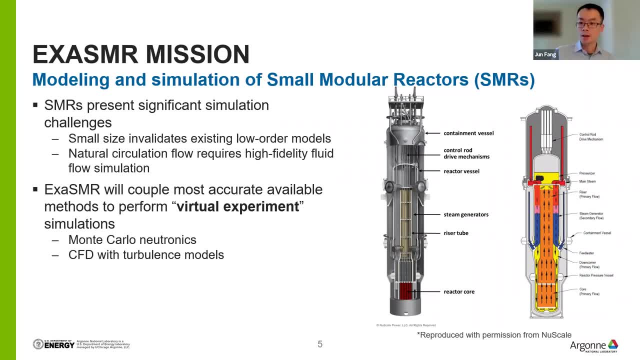 So why we choose the SMR? So it's because it's very different from the traditional PWRs. So first of all, it's much smaller in terms of the size and power, which means a lot. many of the old correlations won't work for this new design. 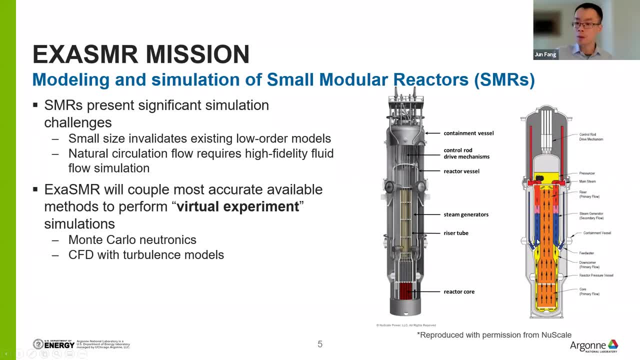 And also, as you may notice, there's no pump in this system, So the SMR is driven by the natural circulation, which requires high fidelity fluid flow simulations. And then here comes the extra SMR. And then here comes the extra SMR. 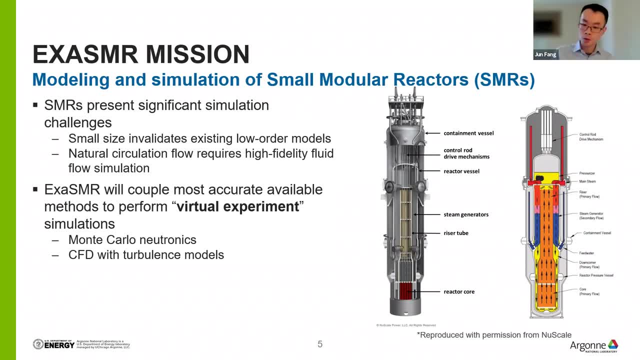 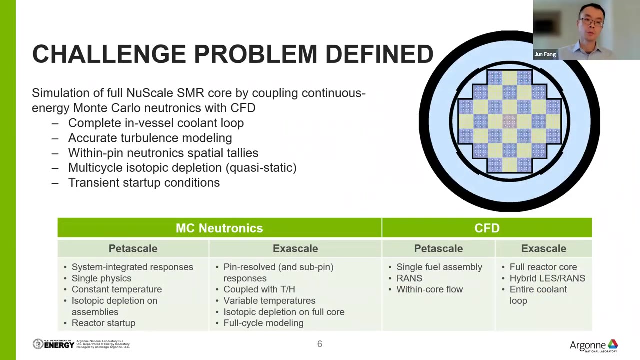 Of which the mission is to couple most available, most accurate available methods to perform the virtual experiment simulations, which includes two primary components- One is the multi-color neutronics And another one is the CFD, with turbulence models And under this extra SMR we define this challenge problem. 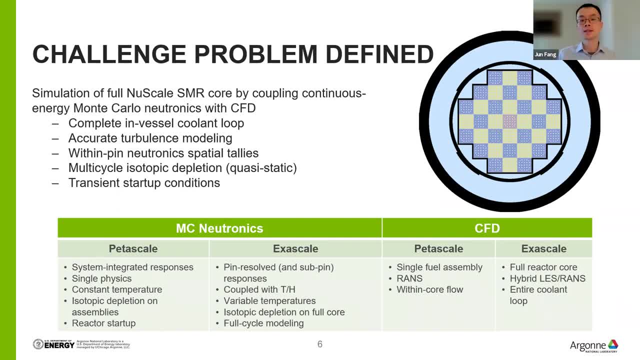 So in order to simulate the full new scale SMR core by coupling continuous energy multi-color neutronics with CFD, we need to have a complete invasor coolant loop. We will need this accurate turbulence modeling and also the capability to perform neutronics calculations at a pin resolved level. 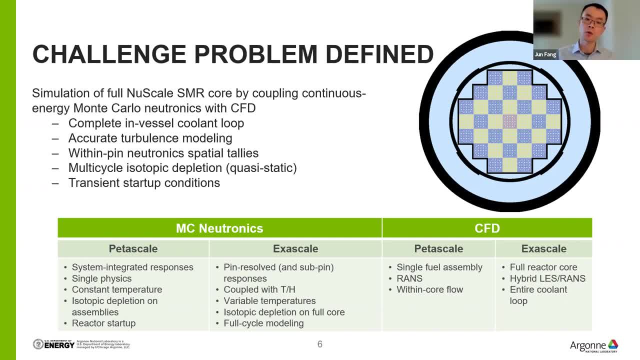 And we also want to study different scenarios, including the quasi-static and also the startup, And in the table on the bottom I just show some examples how the individual physics component can benefit from this upgrade from petascale to exascale. For example, in the CFD simulations on a petascale machine we can only perform the simulations for single field assembly. 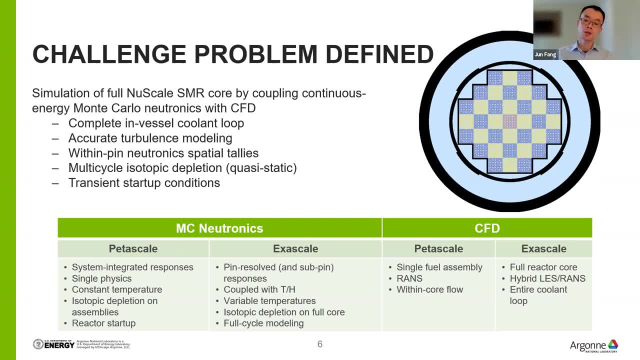 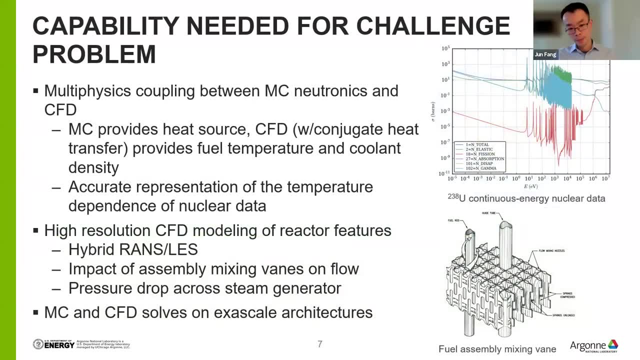 But we can potentially scale that up to a full scale, To a full reactor core on the exascale machine. So here we just summarize the capabilities needed for the challenge problem we're targeting. So first we will need a multi-physics coupling framework between the multi-color neutronics and CFD. 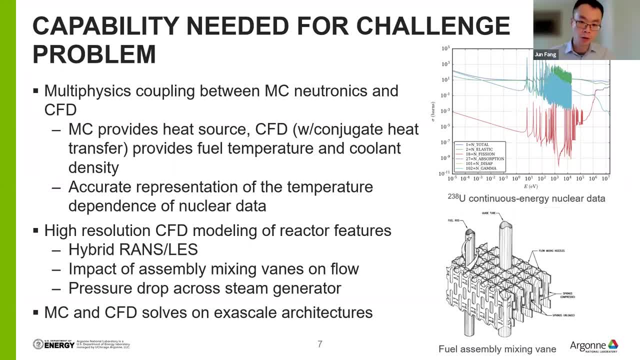 So within this framework the neutronics solver will provide the heat source And the CFD solver with conjugate heat transfer here will provide the field temperature and the coolant density, And we also need the accurate representation of the temperature dependence of nuclear data. 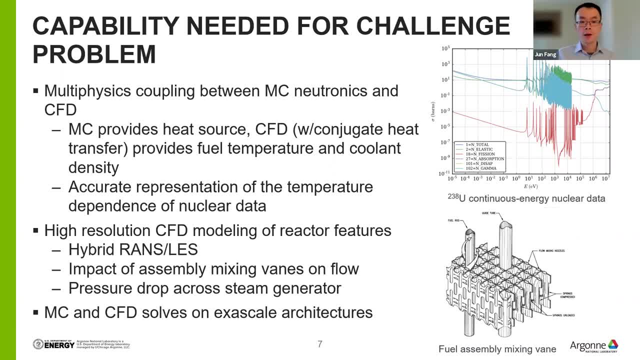 And on the other hand, we also need the high resolution CFD modeling of the reactor features. So one option is to do this hybridization. So, for example, we can do this hybridization for RANS and LES, For example. we perform the detailed, resolved, large-edged simulation for just one assembly within the full core. 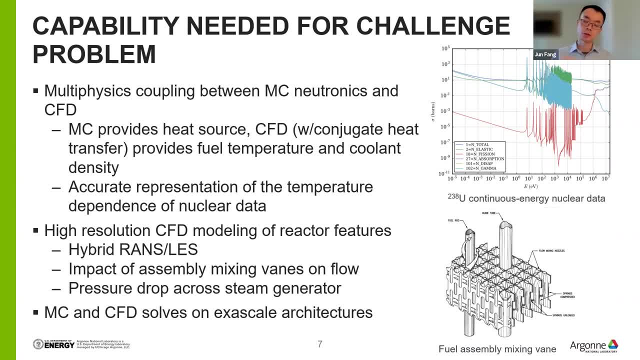 And in the meantime, perform the RANS simulation for the rest of the assemblies, And we also want to include models that will incorporate the effects of assembly mixing events on the flow. As I mentioned earlier, we won't be able to make it. 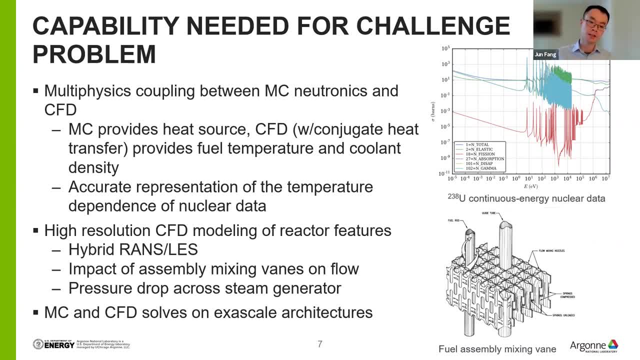 We won't be able to mesh the detailed reactor structures, even with exascale supercomputers, So we will need some models to take into account these effects, And we also want to include the pressure drop models across the steam generator in the SMR system. 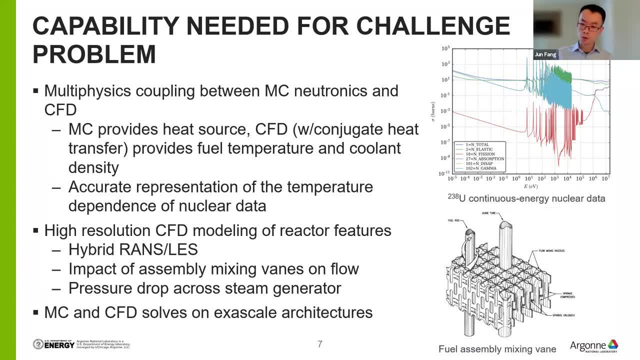 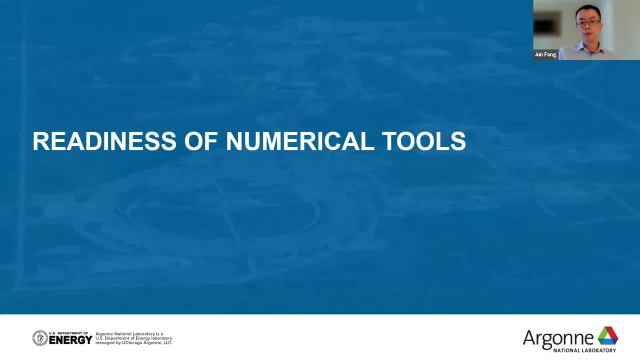 Last but not the least, so we also want to make sure these multi-color neutronics and CFD solvers have one very efficient play on the exascale architectures. So, and in the next section I'm going to show you the state-of-the-art CFD capabilities we have at the lab. 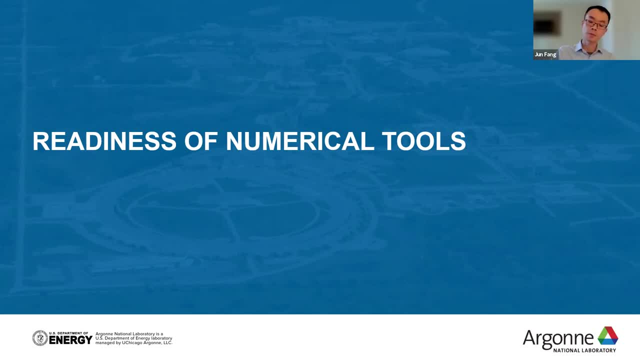 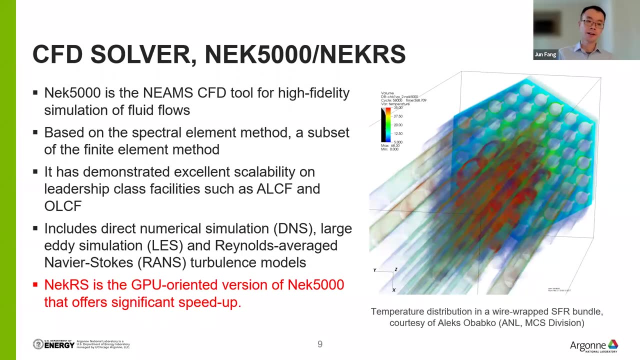 And I will also briefly talk about the coupling framework. So the CFD solver being used in this project is NAC5000 and NAC-RS. So NAC5000 is the NIEM's signature CFD component. It's the signature CFD code for high fidelity simulations of fluid flows. 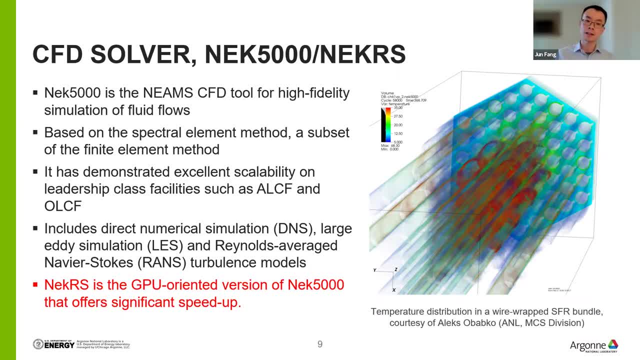 So NIEM's is a DOE program and it's short for the Nuclear Energy Advanced Modeling and Simulation. Both the NAC5000 and NAC-RS are based on the spectrum element method. It's a subset of the finite element which kind of combines the flexibility of domain discretization of the finite element method. 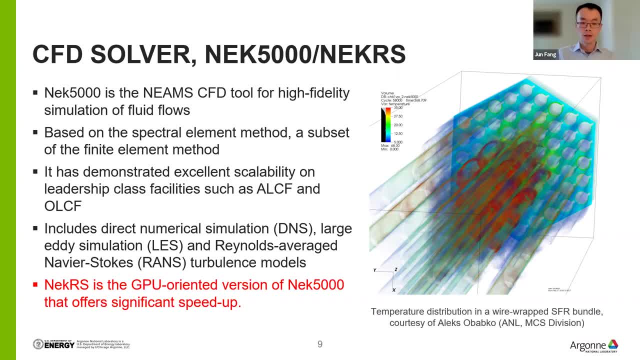 and also the accuracy of the high-order methods. So the codes have demonstrated excellent scalability on leadership class facilities such as MIRA Theta at ARGA and SUMMIT at Oak Ridge. So on the right-hand side, I just show you a nice picture about a wire-wrapped SFRL bundle. 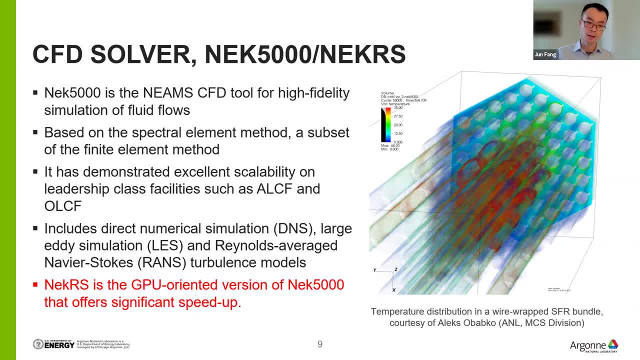 So it's a courtesy from my colleagues at ARGA. So NAC offers a wide range of models, including the high-fidelity direct numerical simulations, large data simulations and also recently implemented RANS models. So I want to mention here for all the new supercomputers being built in the US. 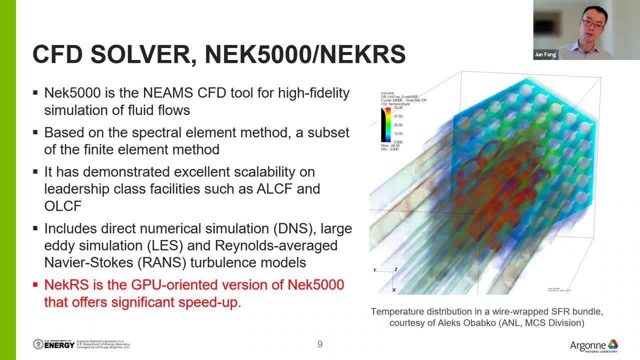 they are adopting a new heterogeneous architecture Which have both CPUs and GPUs. So in order to make the best use of what the new supercomputers can offer, we have to redesign our CFD code. So here we have. as a result, we have got this NAC-RS. 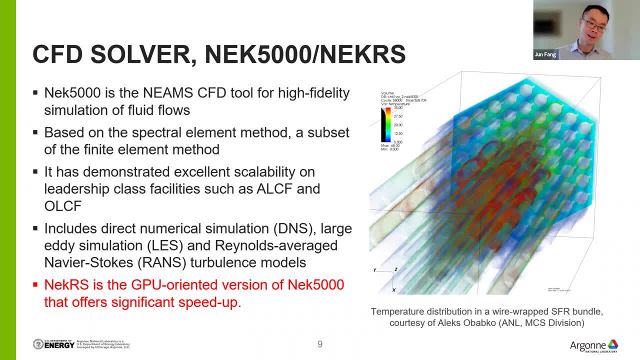 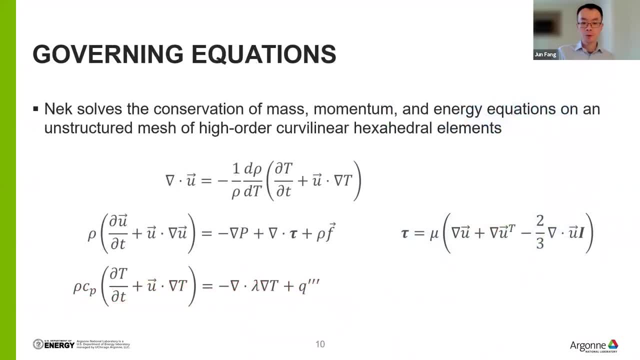 which is a GPU-oriented version of NAC5000 that offers significant speedup on these new machines. So here's some equations. So I don't have a lot of equations in this presentation. So these are the governing equations for the mass momentum and energy conservation equations. 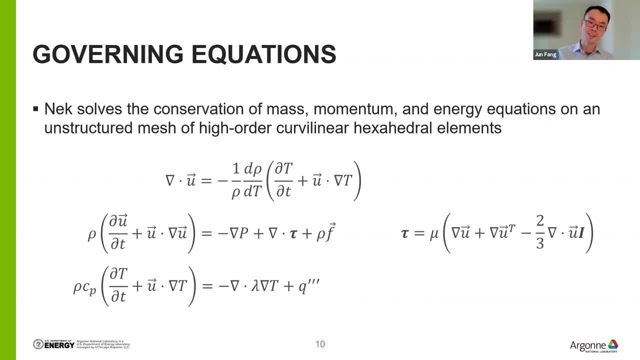 being solved in both NAC5000 and NAC-RS. And here what I show is for the so-called Lohmach number, Lohmach model or Boissonnens model, which will be used in the natural circulation problems. 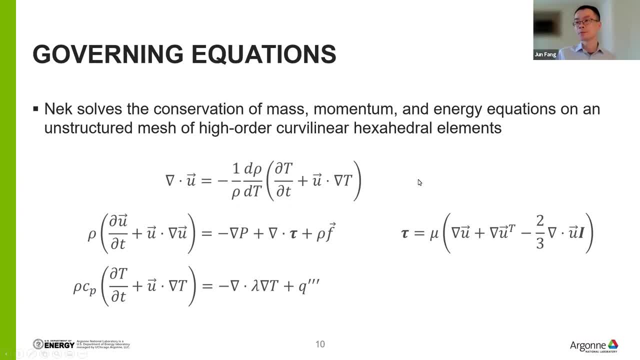 So basically it includes the density dependence on the temperature, And I also want to mention here the temperature is solved as a passive scalar in NAC, And NAC allows you to solve as many passive scalars as you want. So, as I will mention later in this presentation, 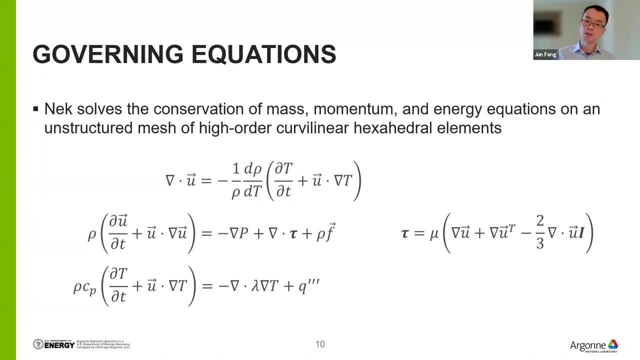 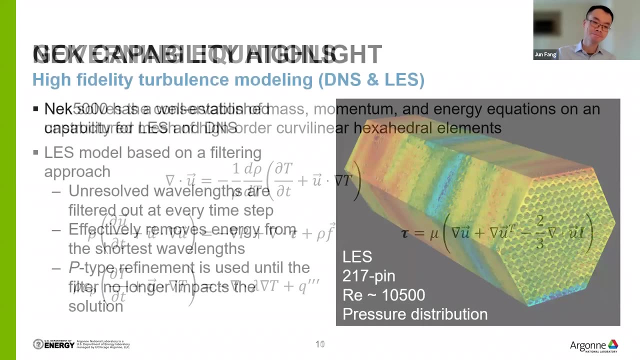 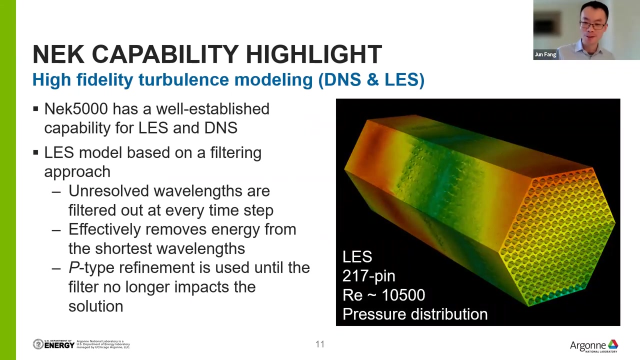 we have the newly implemented RANS models. It's a two-equation K-Omega model. So basically the turbulent kinetic energy and the turbulent dissipation rate are also solved as passive scalars in NAC. So one of the essential tasks in the CFD is to generate the colorful figures and videos. 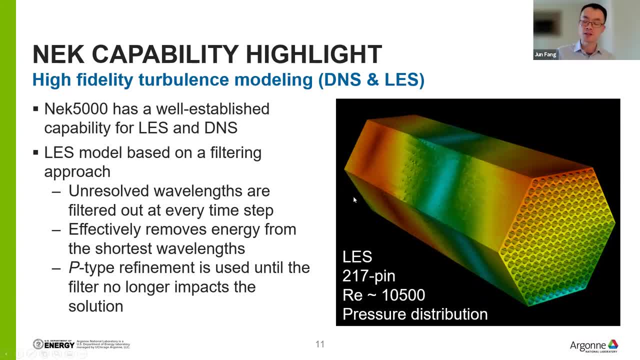 So here is a great example from our LES, the sodium-phosphate reactor. It's periodic in the axial direction and it shows the pressure distribution along the assembly. So basically, NAC5000 has a very established capability for LES and DNS. 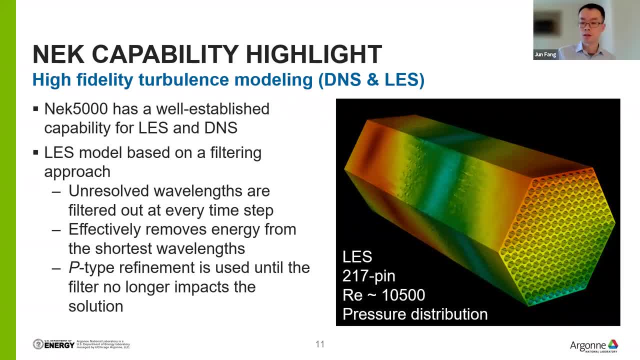 And you can find a lot of journal papers, you know, discussing about the benchmarking and validation of LES simulations or DNS simulations done by NAC, And so specifics for the LES model. NAC offers several different filtering schemes And what I really want to emphasize here is this p-type refinement. 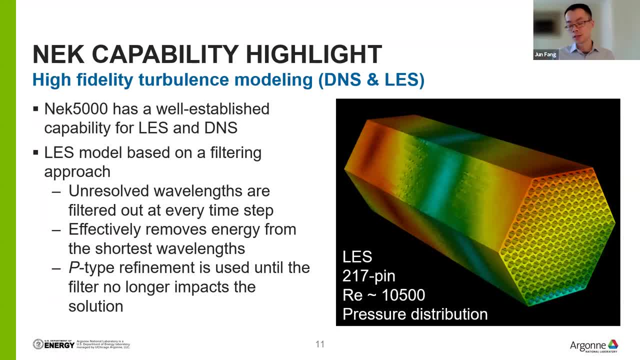 So different from the regular finite element or finite volume codes, NAC has this p-type refinement, which is basically equivalent to the mesh refinement in the finite element, So you can just simply increase the polynomial order and perform the simulations at a much finer resolution. 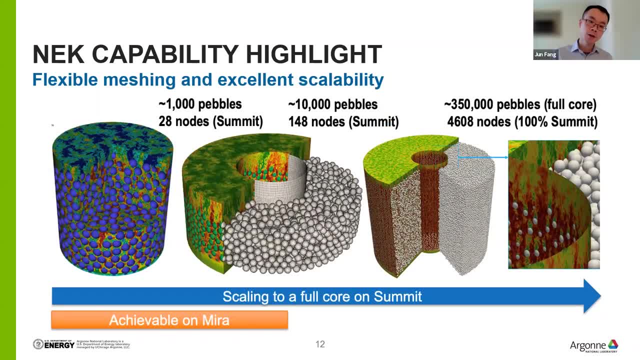 And this is another example to show the meshing flexibility and scalability of NAC. So, as you may know, the paperback is really popular these days and the company X-Energy even got an ARDP award to build their paperback reactors by 2027.. 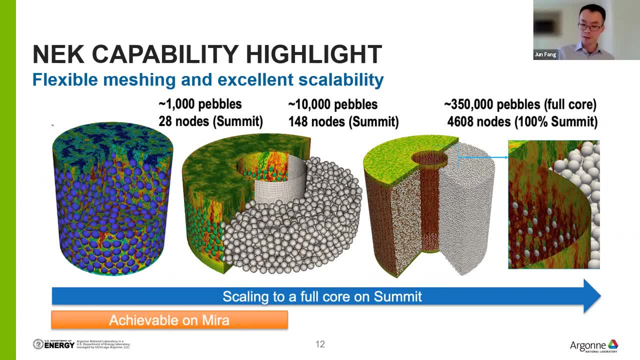 So X-Energy is one of our partners. So in order to accommodate these design needs, we were kind of pushing the limits of CFD, So here we're able to model like a full core of the paperback reactor. 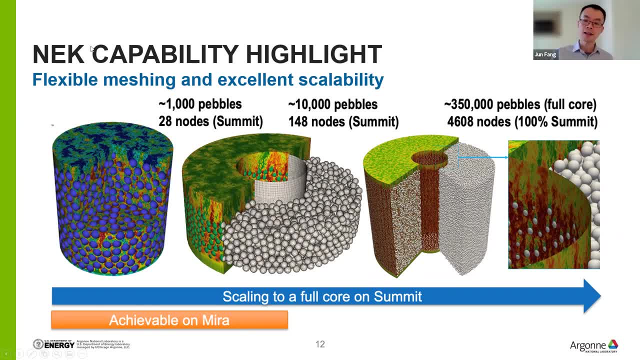 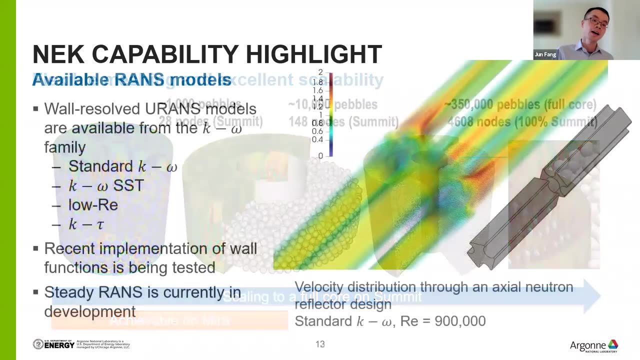 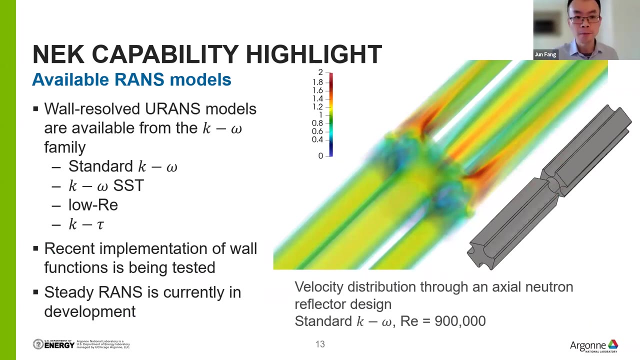 And the code, the NAC, can be scaled up to the entire summit machine. So, yeah, this is a great example to show the scalability of NAC And, in addition to the high fidelity LES and DNS, we also recently implemented the RANS models. 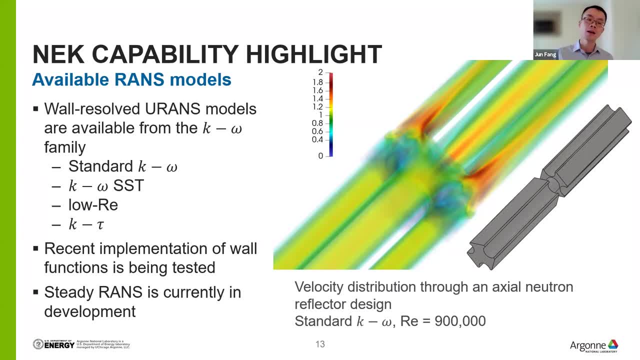 specifically the war resolved unsteady RANS models from the K-Omega family. So currently we have the standard K-Omega, the K-Omega SST, the low Reynolds number K-Omega and also the K-tau model, which is a variation from the K-Omega model. 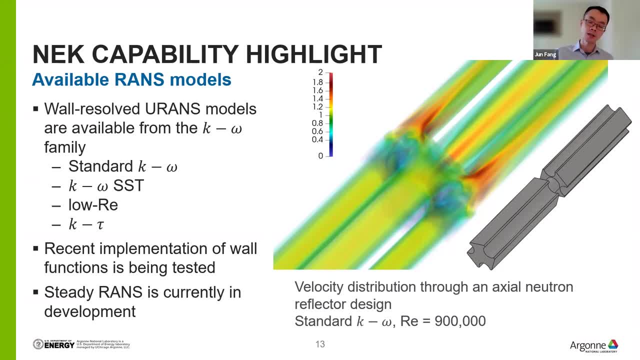 And the tau here is actually the inverse of the omega. And here I show an example: RANS case for the axial neutron reflector design. So the Reynolds number here is very high, It's 900,000.. Talking about the Reynolds numbers, 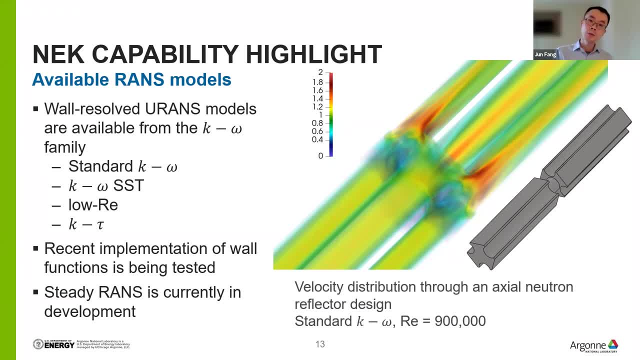 for the typical PWR flow conditions, one can expect the Reynolds number to be about 500,000. in the field road bundle geometry And because the SMR is driven by natural circulation, the flow rate is smaller. So but we do expect the Reynolds number of 60 to 80,000. 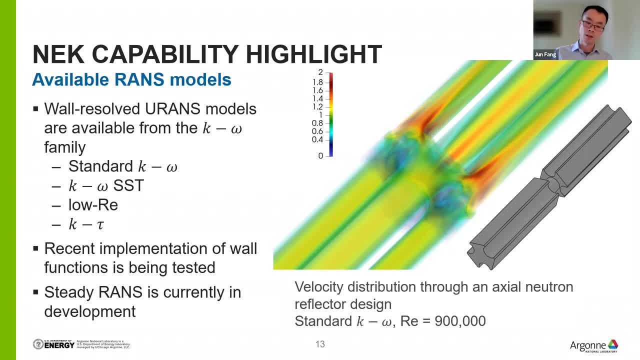 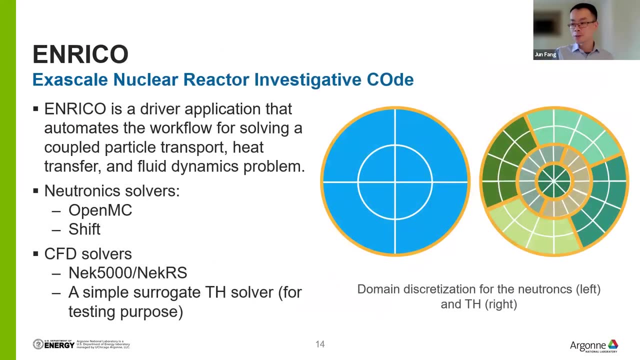 in the field road assembly. So there are also some ongoing efforts to implement the wall functions in NAC, as well as the steady RANS solver. So, in addition to the safety capabilities, I also want to briefly talk about this, our coupling framework. 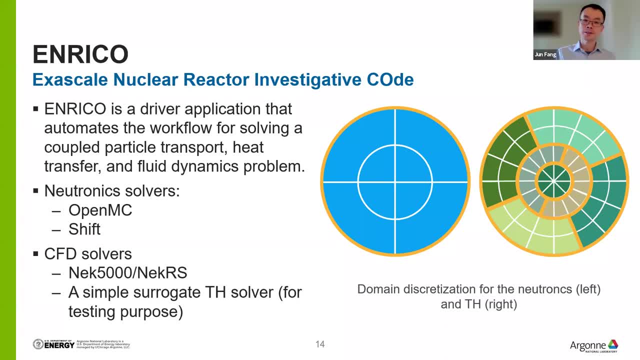 which is called ENRICO, Exascale Nuclear Reactor Investigative Code, So it's also named after our lab funding father, Enrico Fermi. Basically, the ENRICO is a driver application that automates the workflow for solving. 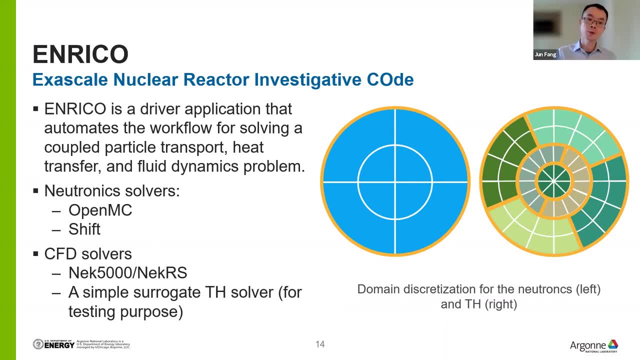 coupled particle transfer, heat transfer and fluid dynamics problems. So here I show two mesh, one for the neutronics solver and another for the TH solver, And so basically, ENRICO requires the two meshes to be conformed. 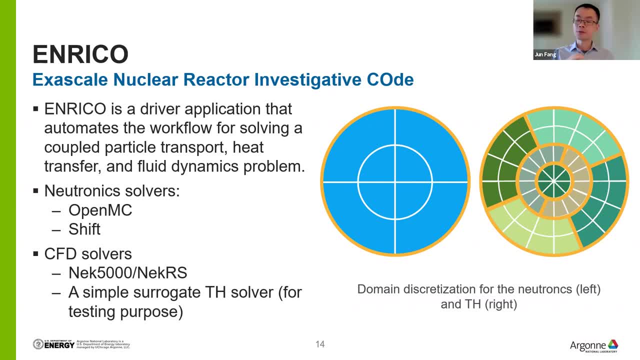 And also it has an efficient communication scheme to exchange the information between the neutronics mesh and TH mesh, Basically like copying the heat source calculated by the neutronics solver to the NAC, and also provide the temperature from NAC to the neutronics. 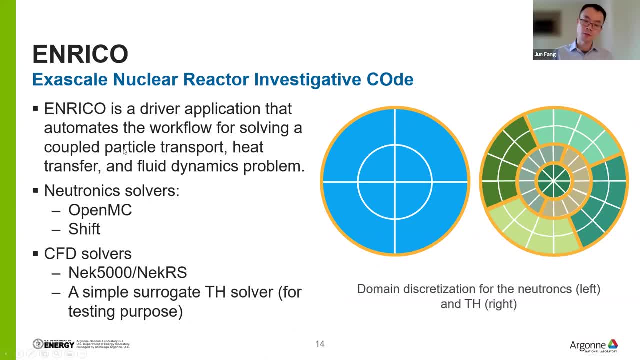 So currently we have two neutronics solvers available: One is OpenMC, another is SHIFT, and at the CFD side we basically coupled the NAC-5000, both NAC-5000 and NAC-RS- to this ENRICO drive. 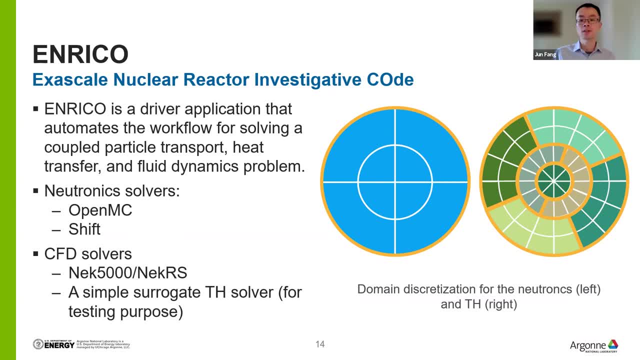 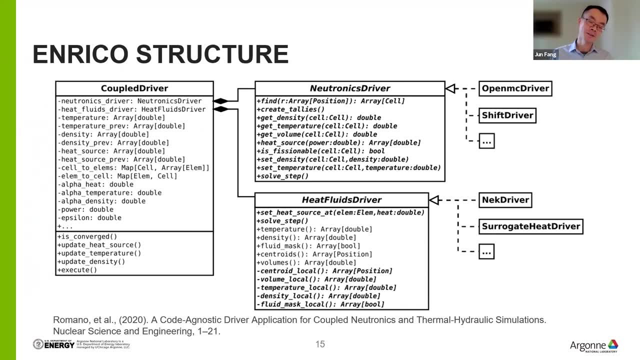 And also there's also a simple surrogate TH model just for testing purpose And here's a like, a detailed structure about the driver application. And so what I want to mention, emphasize here, is that the neutronics, solver and the CFD side. 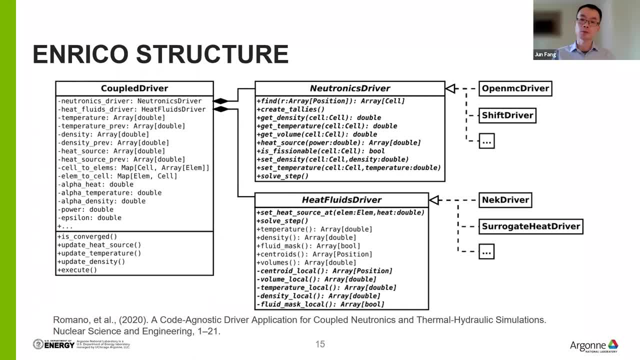 and the CFD solver are coupled in memory, So we don't have to write out any files and then for the communication. And also another strength of ENRICO is its extensibility. Currently we only have two neutronics solver options. 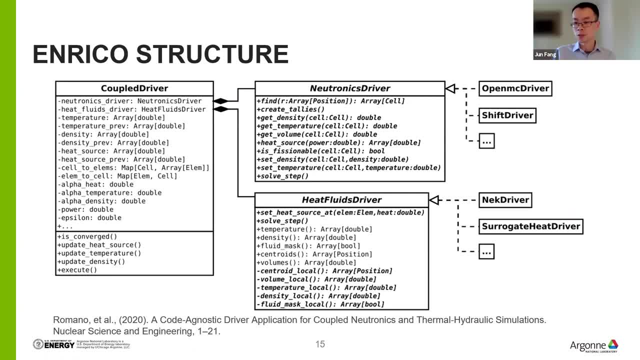 but in the future we can also potentially incorporate other neutronics solvers. So if any of you is interested in this multi-physics coupling driver, you can find a lot of details in the journal paper on the on the bottom. 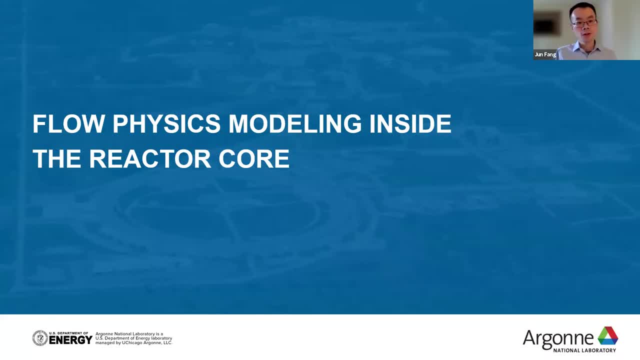 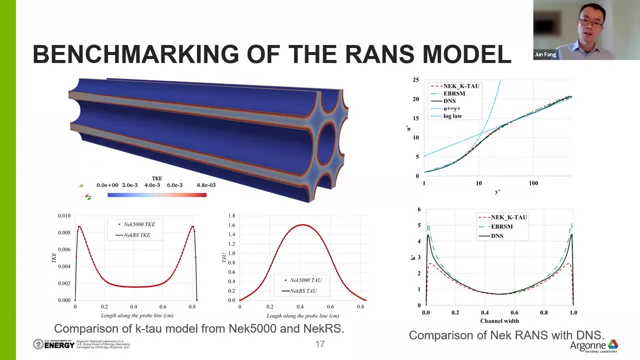 All right, So then we will focus, shift the focus to the full physics modeling. All right, So the the RANS model is relatively new to NAC and also the NAC-RS is basically a new code. Before we conduct: 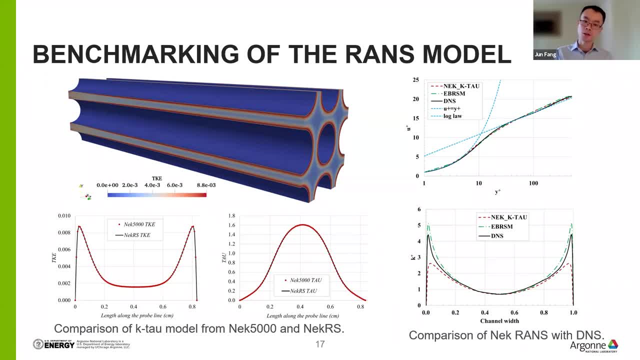 conduct our investigations, we want to first make sure, like the, the codes can give you the right answers. So we did some benchmarking studies. So the first study is to to to compare the results from NAC-RS and NAC-5000.. 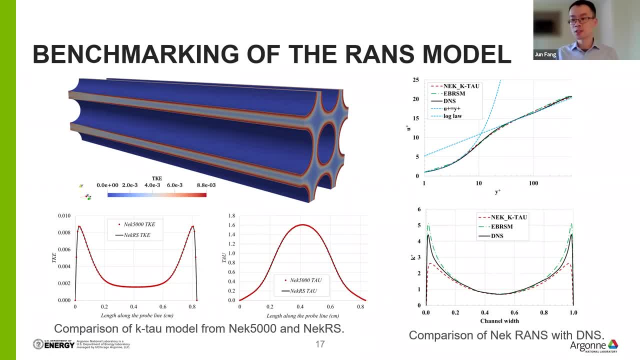 So basically, given the same boundary conditions and input parameters, we want to make sure the NAC-RS can produce the identical results at the NAC-5000.. And and especially for the furor bundle geometry we are interested in. 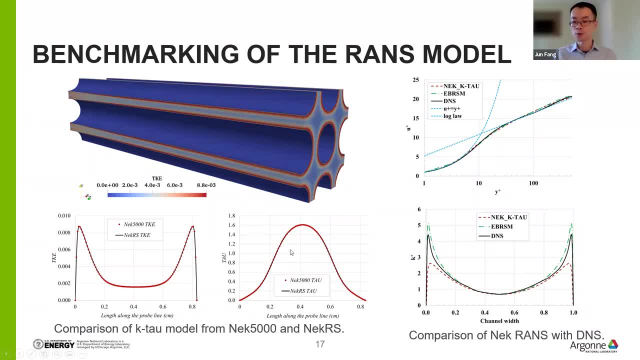 So, and they do have, they do, they do provide these identical results. And at the next step, we also compared the NAC-RS results with other RANS models and even DNS. So, from this law of the wall plot, 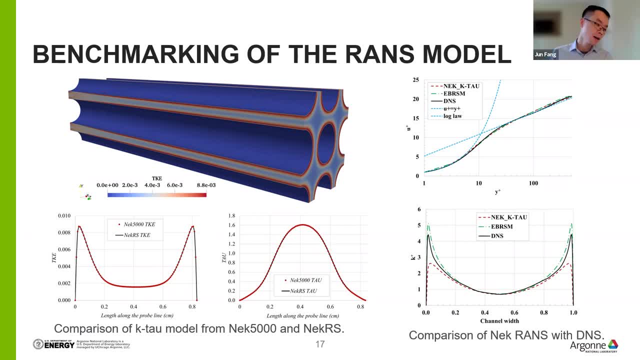 you can see the velocity profile from the from the NAC-RS model agrees really well with the reference data. And as for the turbine kinetic energy, we understand there's there's some difference at the near wall region but overall the 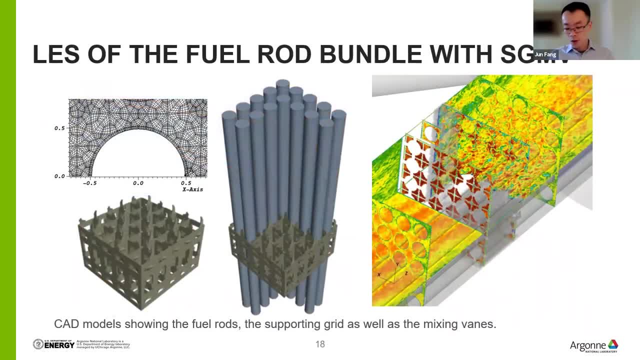 the accuracy is good enough. So in order, so in the, in the real nuclear reactor core, like within the assembly, we have these detailed structures. So one of the most important geometric features is the. is this spacer grate which? 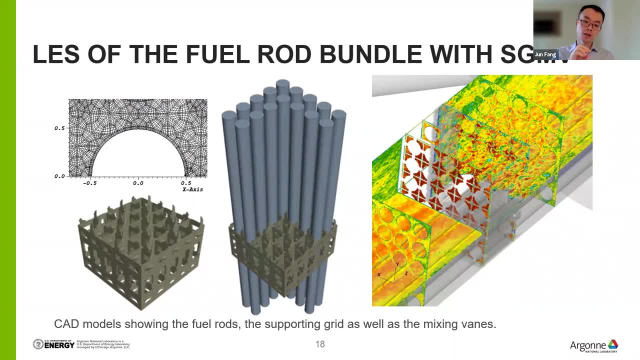 which is used to hold a few rods together, And also the. the mixing vanes are installed on the spacer grate to promote the flow mixing and thus improve the convective heat transfer inside the core. And so, in order to model this, the influence of this detailed. 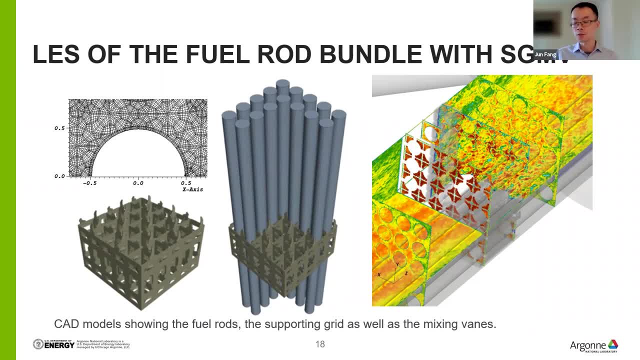 geometric structures, so we need to develop some dedicated momentum sources. But in order to develop the develop and calibrate this momentum sources, we need some reference data. That's the reason we perform the large eddy simulations for this geometry. So in the figure 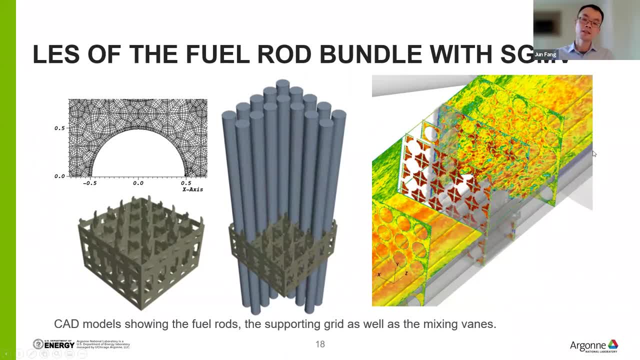 on the right hand side you can see the strong influence from the mixing vanes. There's a lot of flow rotation downstream the spacer grate. So we we perform the large eddy simulations as as to to generate the reference data. 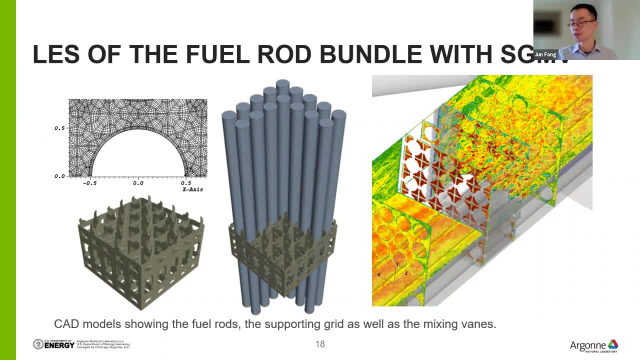 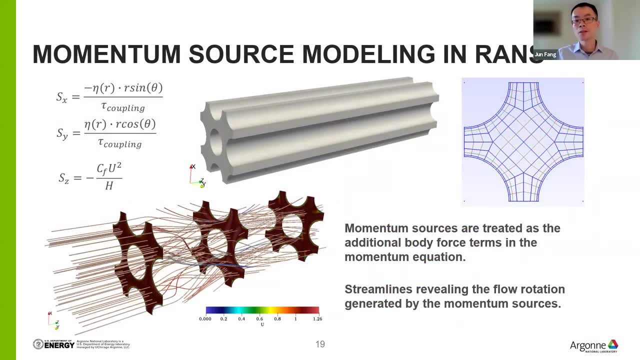 and then use this data to calibrate the RANS models, the momentum sources in our RANS models. So, talking about the momentum sources, the the formulation we proposed actually are very simple. So there are two. there are two important parts. 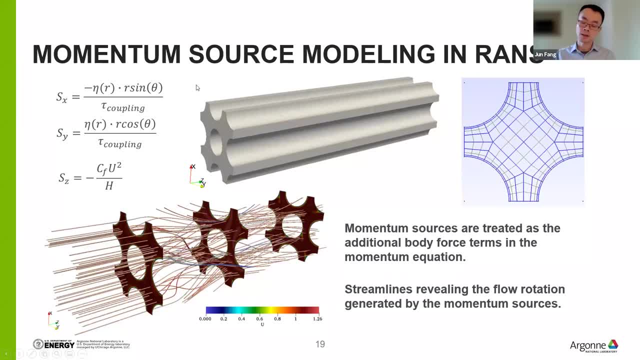 One is this eta and another variable is this coupling time scale. So basically we will use the LES data to tune our eta. So for the RANS case, I also show the discreditation of the of the domain for a single sub channel. 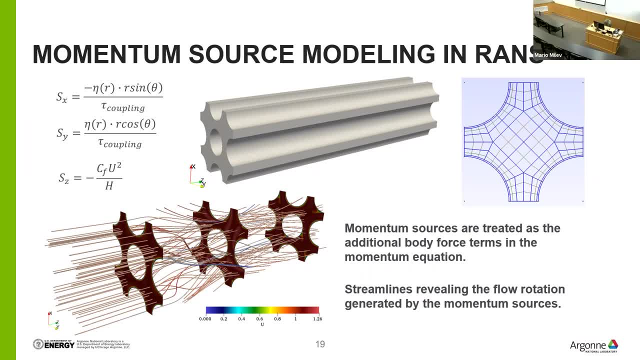 As you can see, the mesh is much coarser than the LES case, which allows us to scale up the simulations And on the bottom, by applying this momentum sources, you can see this kind of twisted streamlines in the in the fuel bundle. 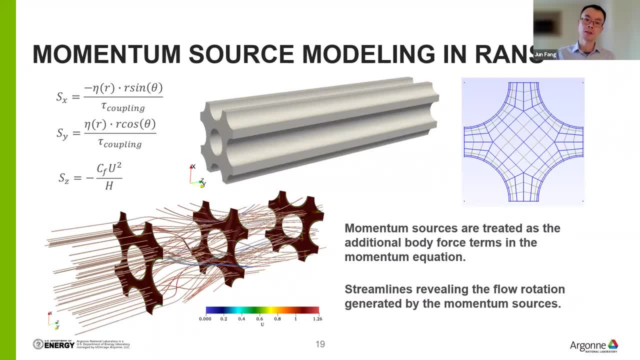 which is a clear sign of the effectiveness of the momentum sources. But we'll also have to make sure we we reproduce the right kind of, right level of flow rotation in the domain, as we observed in the LES with the resolved geometric details. 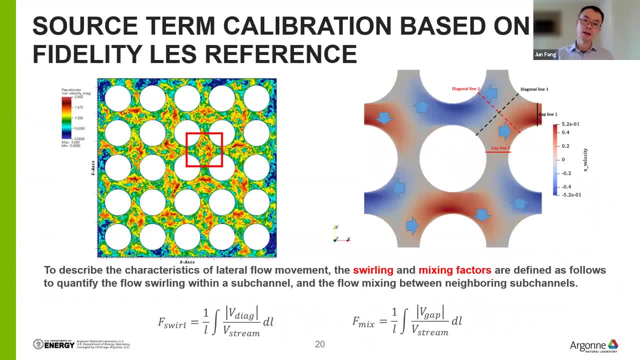 So then, how we characterize the, the flow rotation or the effect of the mixing lens in the in the LES case. So to your. for that purpose we define two important quantities: There's a swirling and mixing factors. So one is used to. 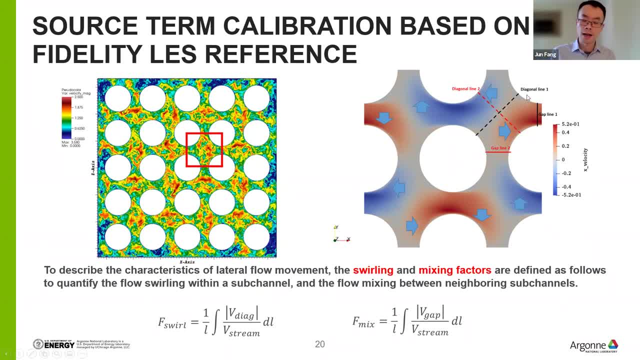 so basically, the, the swirling factor is the averaged the crossflow magnitude along the diagonal lines here. So basically, this quantity is a good indicator of the flow swirling within a sub channel And the mixing factor is the averaged crossflow along the across the gap lines. 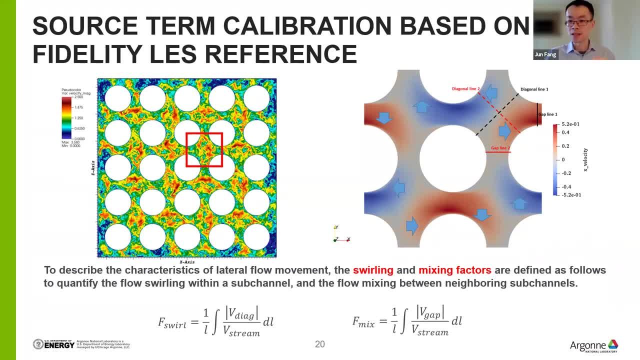 which is an indicator of the crossflow between neighboring sub channels. So so this way we can extract some quantities and use that quantity to tune our momentum sources and make sure we can reproduce the same level of flow rotation in the RANS case. So here, 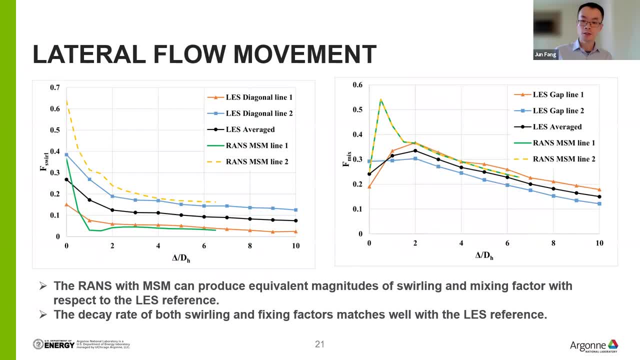 here are some results for the swirling and mixing factors and and the comparison between the, the RANS and LES case. So as you can see here, the, the- the RANS case with momentum sources can produce the equivalent magnitudes of the swirling. 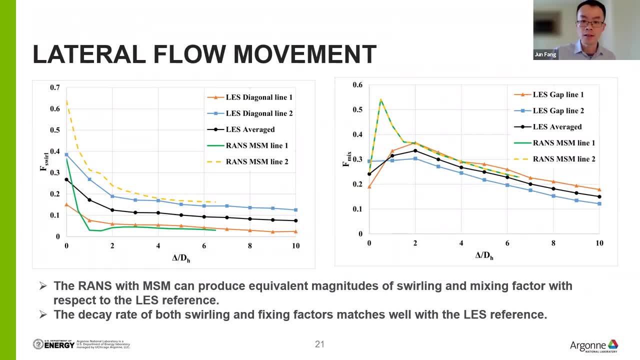 and mixing factors. There is some division at the beginning of the of the application momentum source application zone, which is expected because in the in the real design, a lot of space is occupied in the in the real reactor assembly, But here in the barrel. 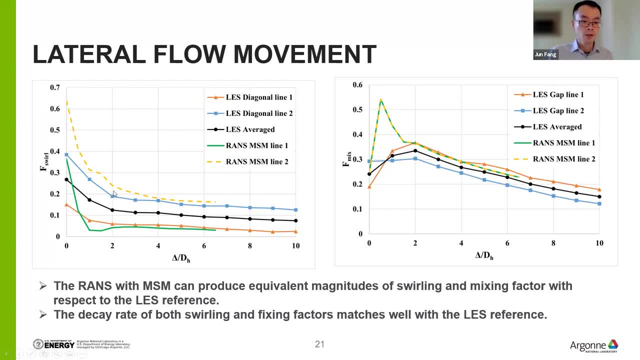 barrel bundle. we don't have that. And also, in addition to the magnitudes, we'll also the momentum. sources developed are also capable to capture this decay trend, like how the how the effect of mixing vanes reduce in the downstream location. 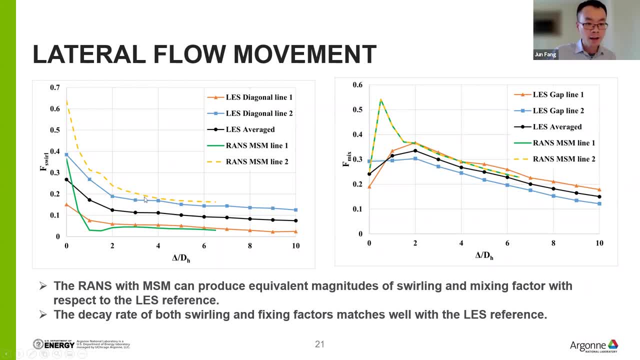 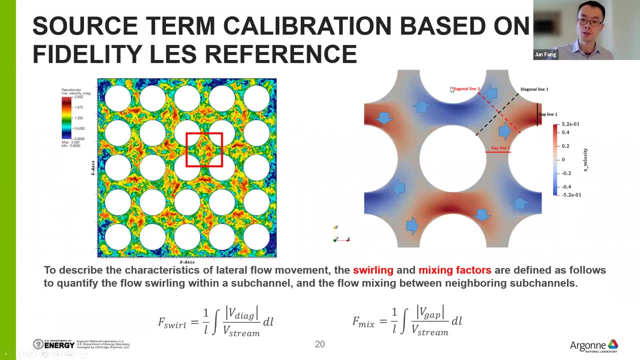 at downstream locations. So here, as you may notice, the the, the movement factors along two diagonal lines are significantly different. That is actually related to the specific deflection of your mixing vanes in a sub channel. So they they have this altering pattern. 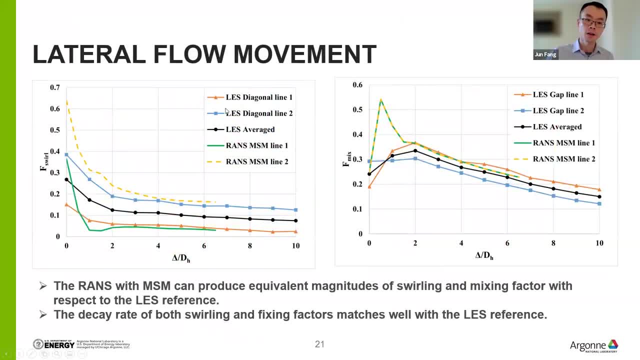 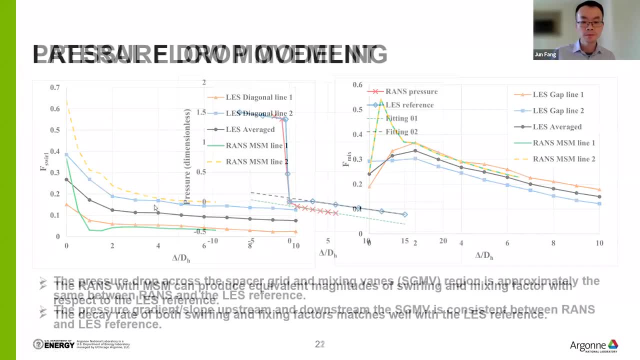 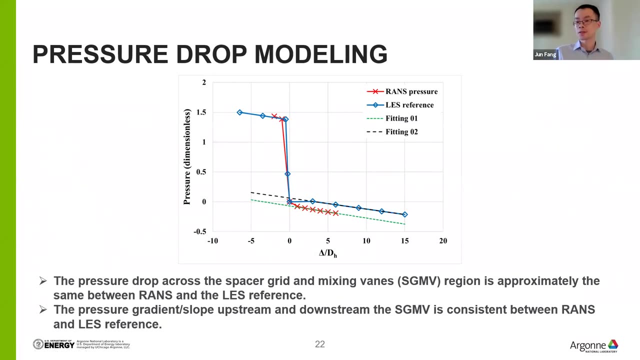 for the deflection of mixing vanes and the mixing. So and the moment. we're glad the momentum sources can also capture that subtle difference. here And in the string wise direction, we also want to reproduce the pressure drop, because it's very important. 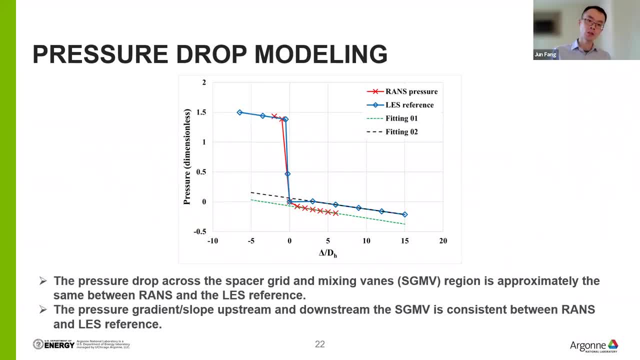 And it. it determines the overall flow rate in in the SMR system. So by tuning our momentum sources we're also able to reproduce approximately the same pressure drop between the LES, between the RANS and the LES reference. And, more importantly, 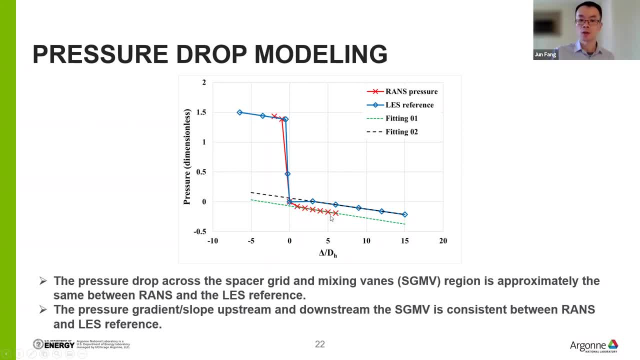 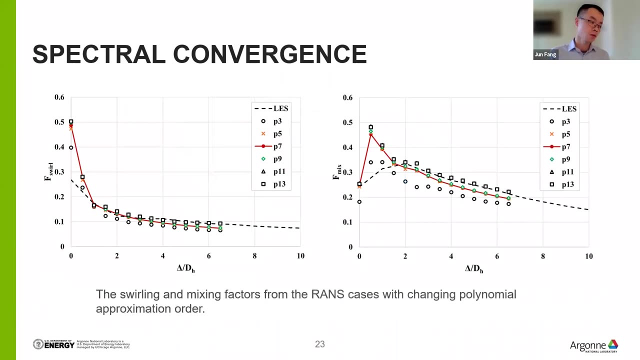 the, the slope of the, the pressure or the pressure gradient are the same or very close downstream, the, the spacer grade region. So for the spectral element method we also want to do the mesh study to to see how sensitive the momentum sources are. 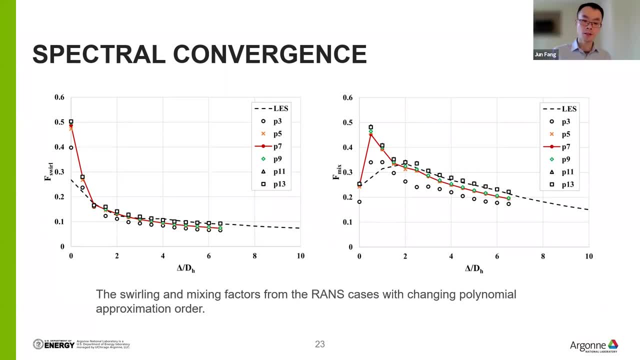 respect with respect to the mesh simulation resolution. So here, as you can see, with a very low, with a low polynomial order, that is, core, relatively coarser mesh, we see larger deviation from the LES reference. but but by increasing the polynomial order, 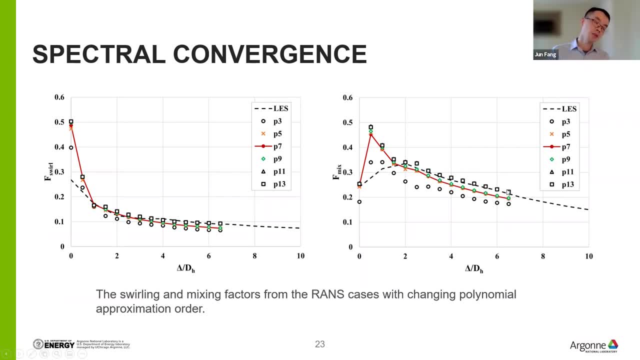 we're able to, you know, make the RANS results converge to the to reference data. So here the, the, the actual polynomial order we, we choose is actually the, the order of seven, which is actually the. actually a sweet spot of NEC. 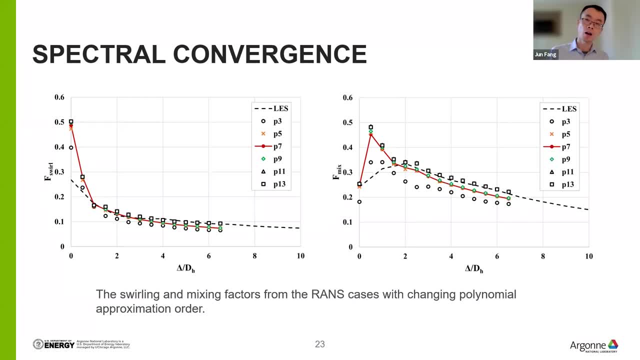 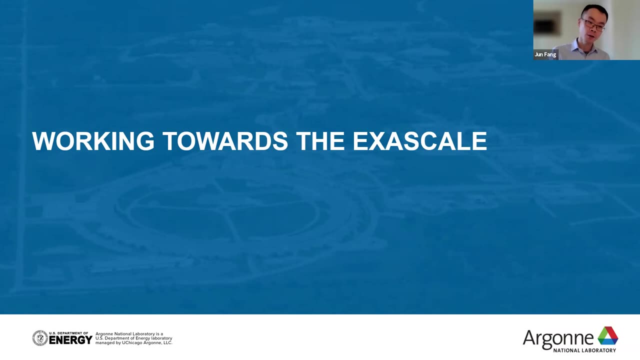 where NEC can deliver, like optimized efficiency And also. so it's a kind of a balance between the efficiency and accuracy here. So, and in the next section I will talk about our recent efforts by pushing this CFD capabilities and coupling and coupling framework. 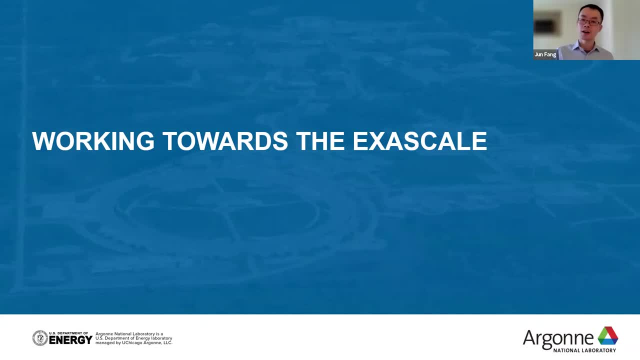 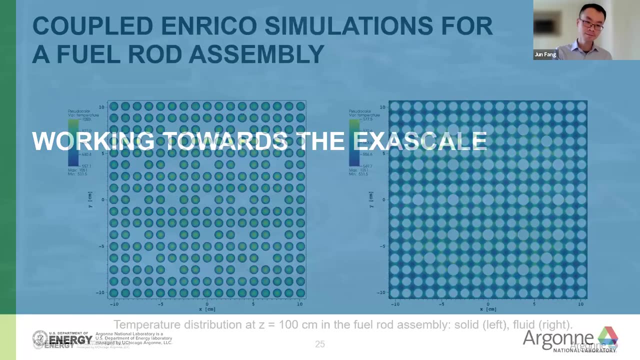 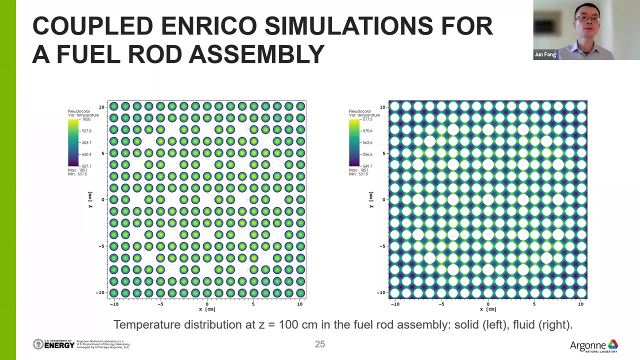 and to the applications of a full core, full core SMR and also make sure they are ready for the X scale. So here, so here I show the some temperature fields from the coupled, coupled simulations for just a few few rod assembly. 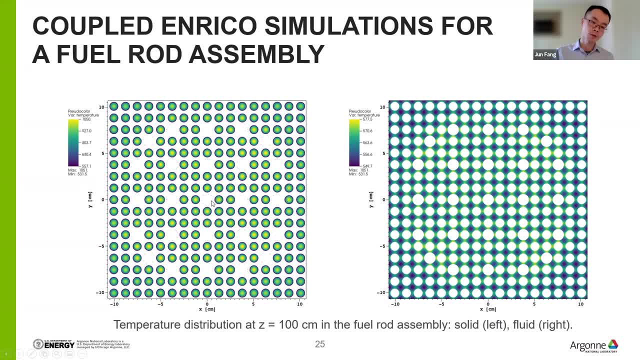 So here on the left you can see the, the temperature from the solid region, which are the, basically the few rods, And the the empty spot here are actually the locations of the control rods, And on the right hand side I show the temperature distribution in the fluid region. 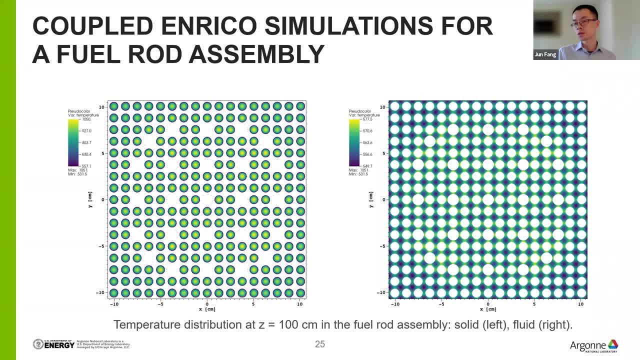 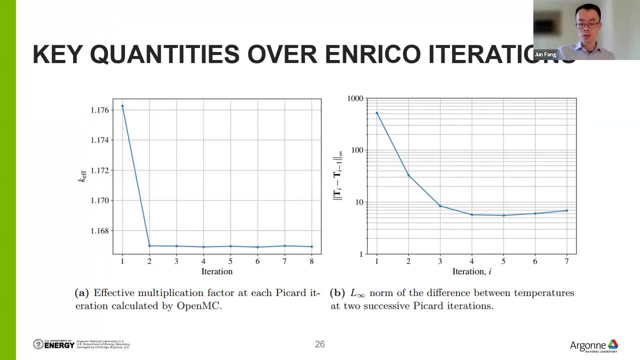 which is for the coolant. So we observe a peak temperature of about 1050 K in the in the in the few region and overall like about 50 K, about 50 K temperature rise for the coolant. Here are here are some other key quantities from the coupled simulations. 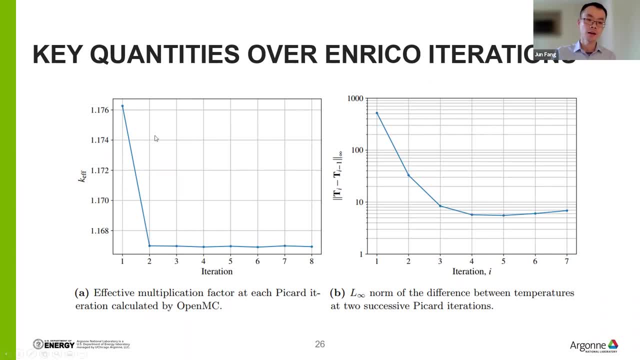 Why is the key effective? So you can see the: Enrico quickly converges, converge over the iterations. So Enrico actually performed this so-called Picard aberrations to, to the conversions. And then on the right hand side, I just show the: 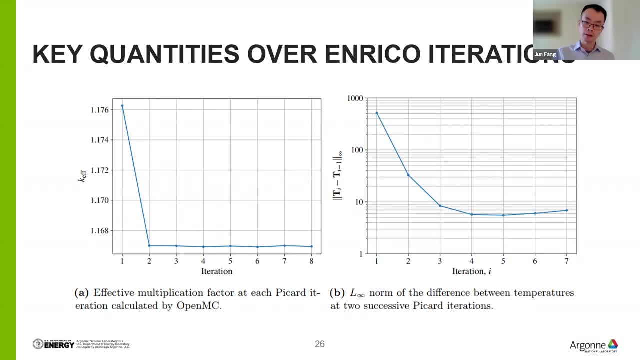 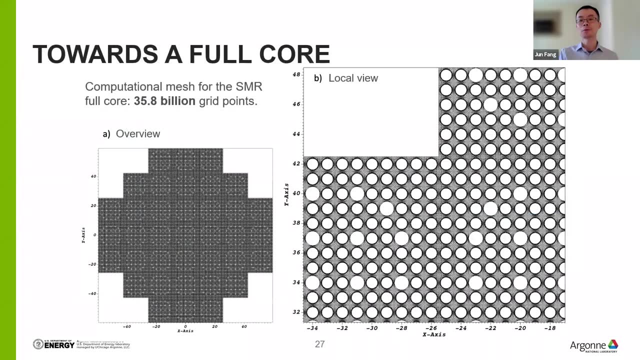 the change of temperature at every iteration. Then we move forward. We want to cause the goal. the goal is to be to be able to perform the couple multi-physics simulations for full SMR core. So so here I just show the mesh for the 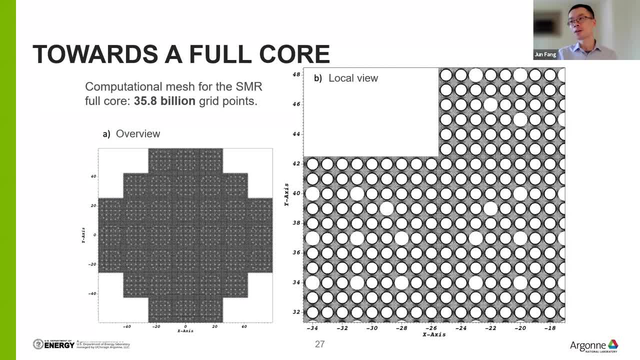 for the full core For SMR there are: there are 37 assemblies in the core and each core consists of, and each core head is basically a 17 by 17 road bundle, So it's a huge mesh which has about 36 billion degrees of freedom. 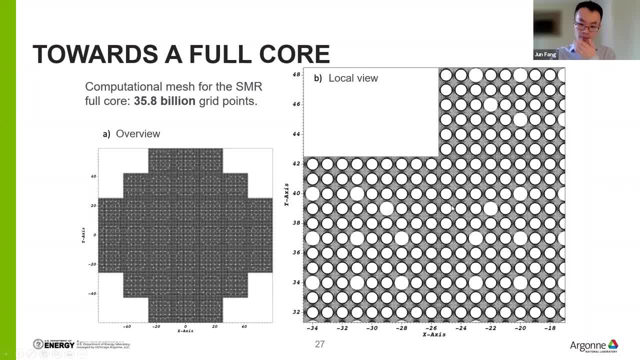 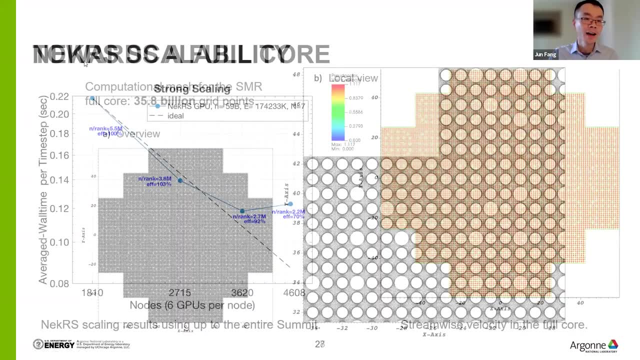 So here there's a local view for the mesh and you can see the, the regular circles for the, for the few rods and also larger circles for the control rods. And here I only show the, the fluid domain, And we also did a scaling study for the. 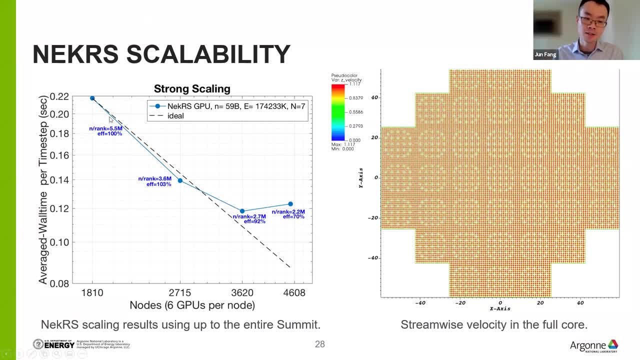 for this full core MSR case, As you can see, as you can see the next skills really well, up to the full core, up to the entire summit, And at the entire summit, we still have 70% parallel efficiency, which is: 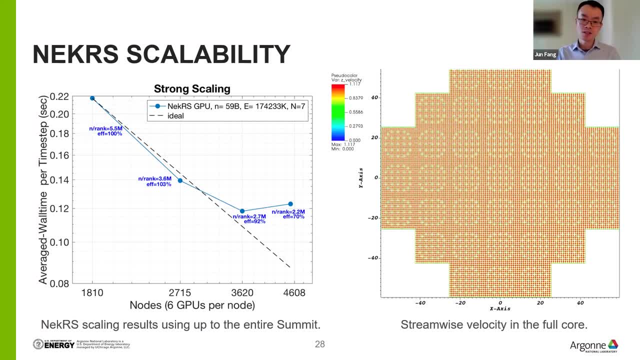 which is good. But I also want to mention NECRS is still under active development and we expect better scaling results in the near future. And on the right hand side I show the the distribution of string wise velocity from the full core. It's because it's the domain is so large. 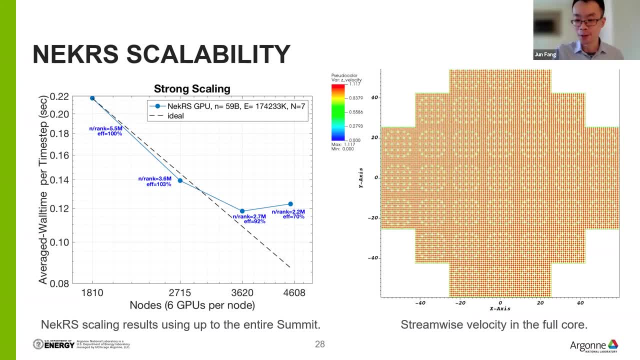 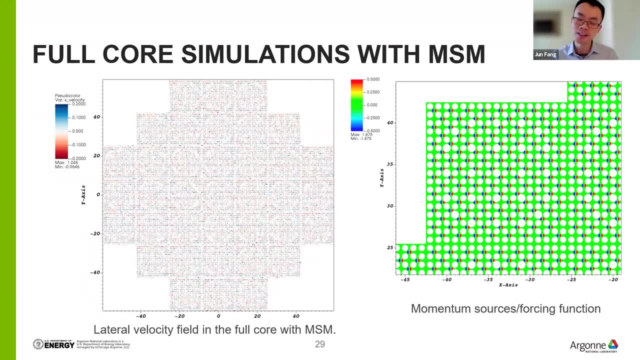 kind of a little difficult to see the local data. So to see the local details, And here we also try to apply the momentum sources, in the full core And on the right hand side you can see the distributions of these momentum sources or forcing. 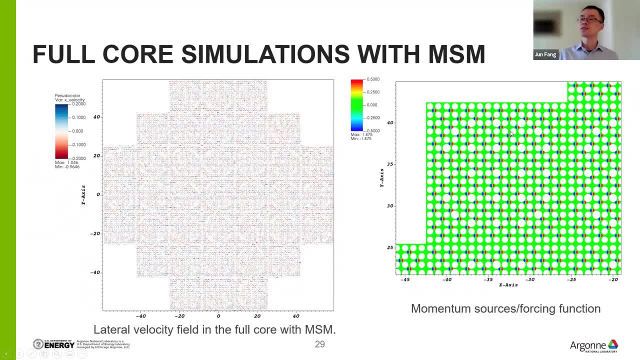 functions. And I also want to emphasize the some of the nice flexibility about this. momentum sources, For example. you can decide whether or not to apply the momentum sources around the control rods Or in the edge channels of the assembly, And you can also decide 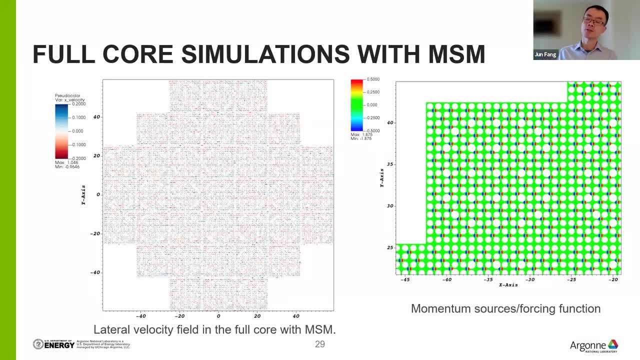 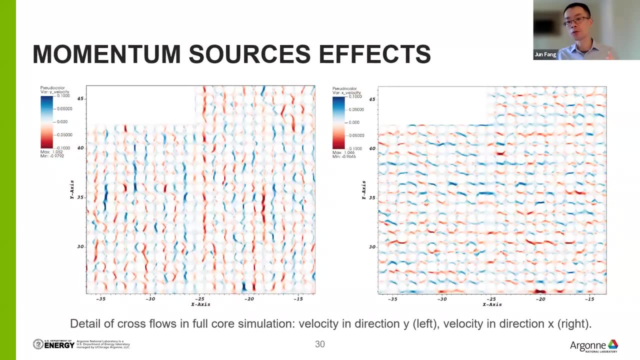 How many layers of momentum sources you want to have in the vertical direction, because in the in the rear nuclear reactor you have multiple layers of space of grid along the span of a few rods. And here's a local view of the crossflow in the: 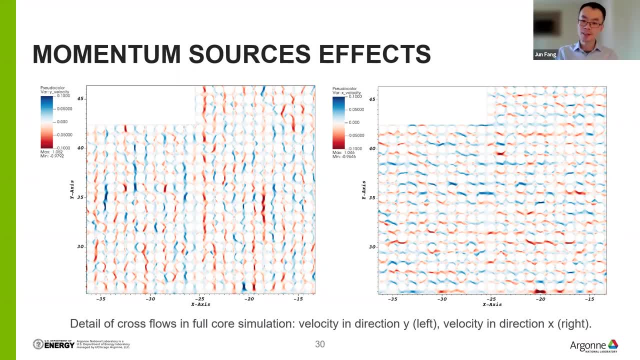 in the full core from the full core simulations And then you can see there are strong crossflows Generated by the momentum sources, which is promising And of course, we will do Like more testing of this momentum stores application in the full core. 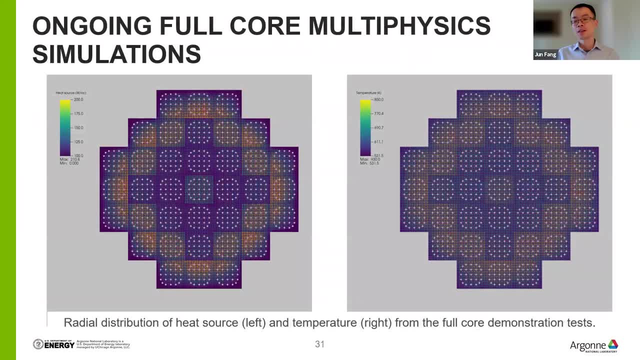 In the near future And here. So what I have presented before only from the, The full core results are only from the CFD, only simulations, And most recently, we're trying to extend the capital, We're trying to extend the modern physics simulations. 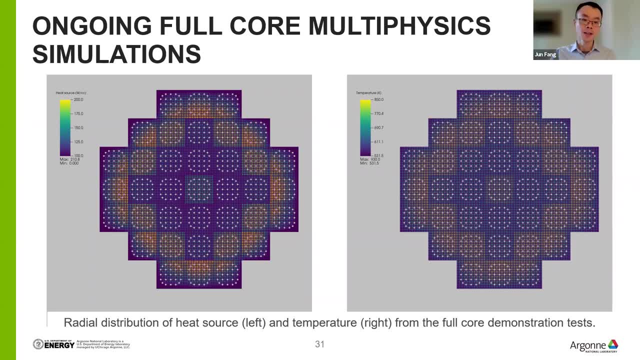 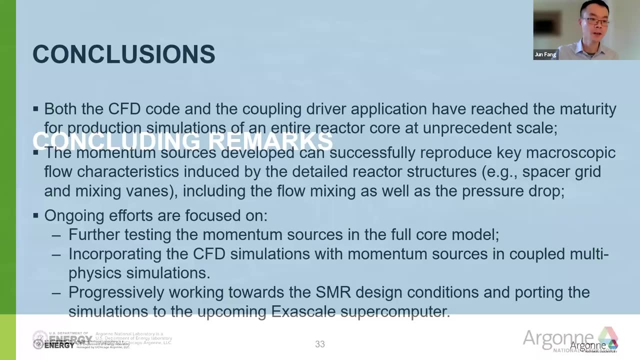 To the full core as well. So Here are just some early results from the this effort, And we show the the heat source and temperature field from the full core. Well, that's about it. So, in conclusion, Both the CFD code. 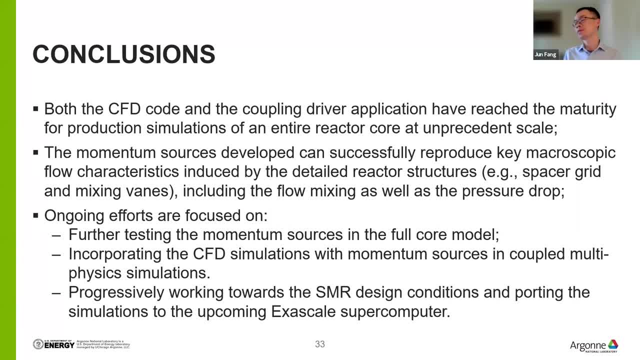 And the copying driver application have reached the maturity For production simulations Of an entire reactor core. So in other words, So these capabilities Already ready for For simulations on the new access scale supercomputers? Hopefully we will see them next year. 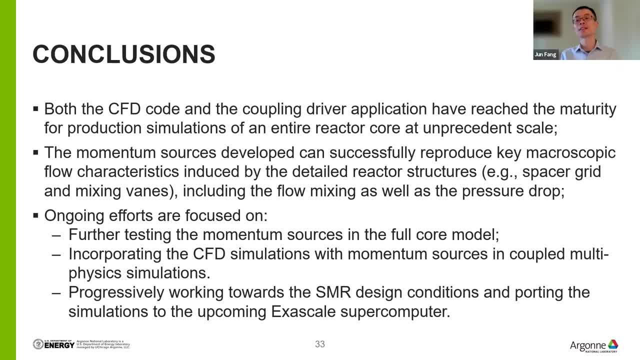 And in the meantime, the momentum sources we developed can successfully reproduce the key Flow characteristics Induced by the detailed reactor structures, such as the space of grade and mixing events. So we can reproduce both the Flow movement On the lateral or cross sectional plan. 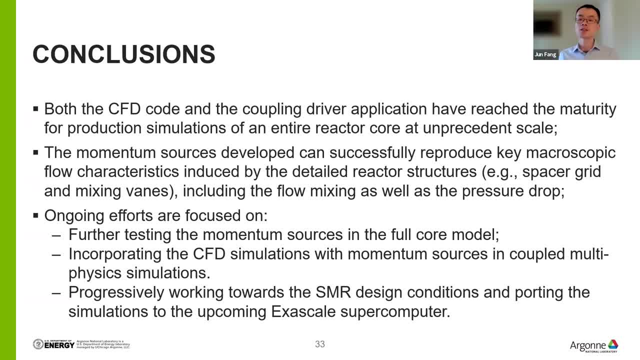 as well as the pressure drop in the stream wise direction. So, as a walk in progress There are there are also a lot of efforts going on right now, So We were testing the momentum sources in the in the full core model. 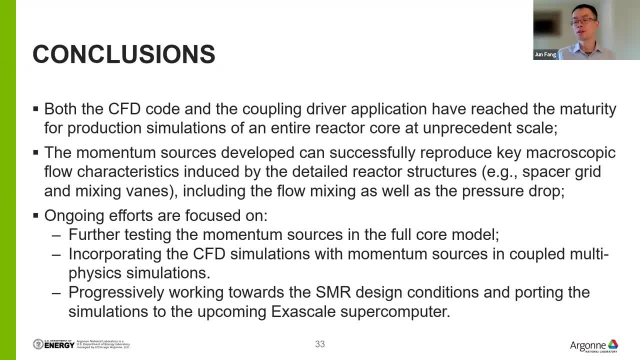 And we also want to incorporate the momentum source For the coupled model physics simulations And eventually we want to Progressively working towards the SMR design conditions. So for the simulations, you, you, you have seen the Reynolds number. It's actually only. 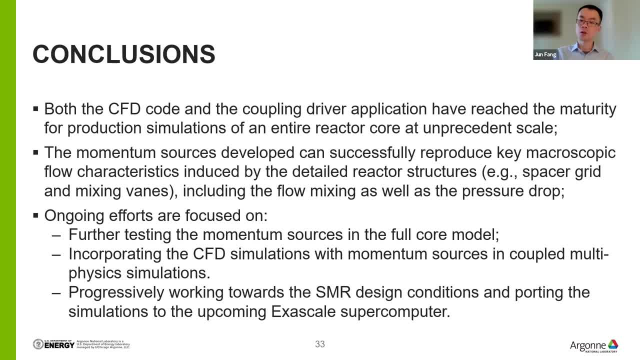 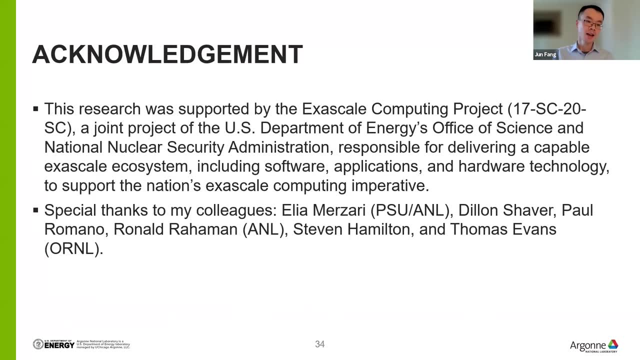 Like about 10,000. Which is still slower from the expected value of 60 or 80. Thousand. So we also want to port these simulations to the New supercomputers. So again I want to Acknowledge the the research I presented. 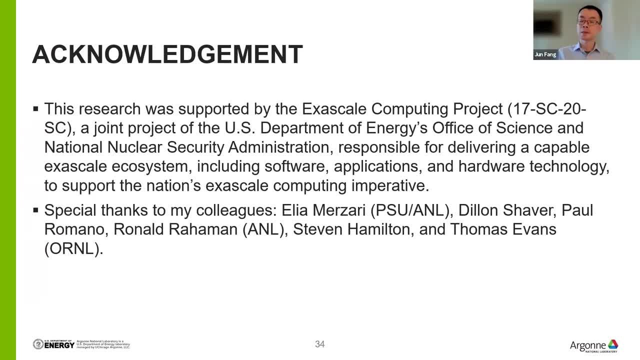 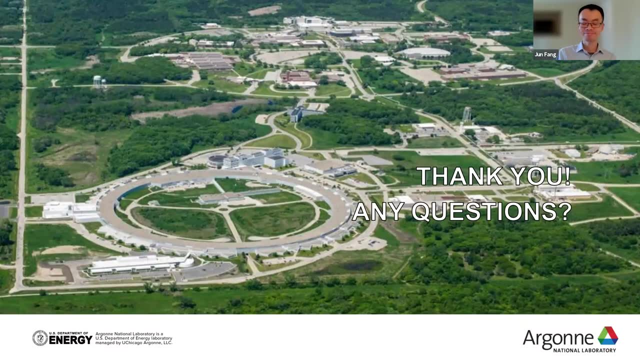 Is funded by the access to your computing project And also it's a teamwork, And I was. I want to give special thanks to my colleagues from PSU Argonne and Oak Ridge. So thank you for your attention And I'll be glad to answer any questions. 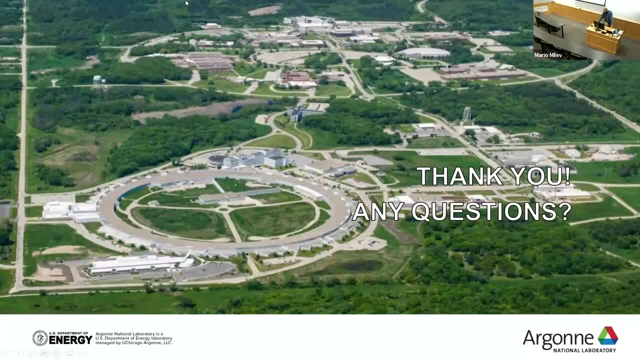 All right. Thank you very much For a great presentation. So we're going to- we're going to queue up the chat here And also, if the participants would prefer to ask their own questions, Please feel free to raise your hand and I can call on you. and feel free. 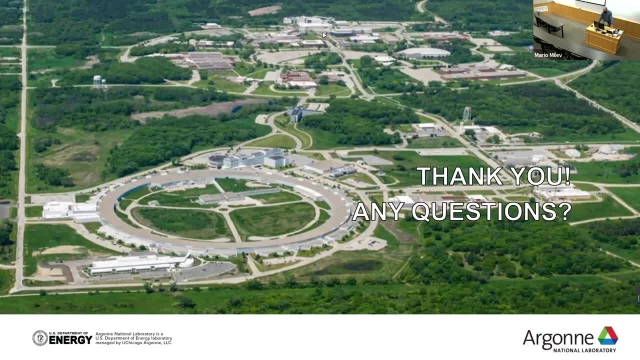 to ask a question yourself if you'd like. So first off, Is there any questions from any of the In person participants Before we get started? Okay, We're waiting to see if. if anything comes up, I'll start asking some of the questions in the chat. 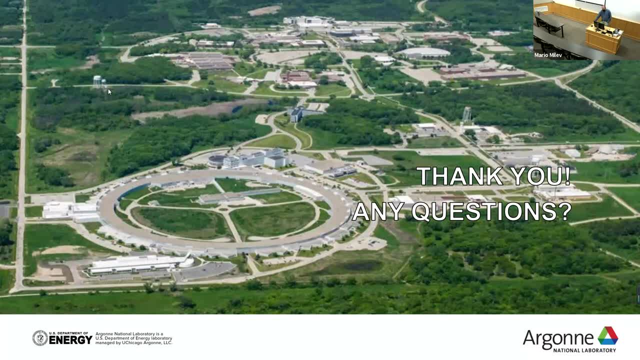 First question from Patrick Hartwell. So what level of precision Is exascale referring to half, single or double precision? So it's double, I think for a half The summit can already, You know, Perform the exascale, you know. 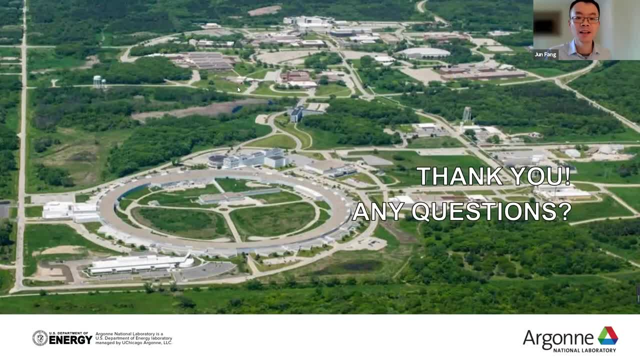 With half precision. Yeah, Okay, It looks like Dr Bolanoff also clarified. Oh yeah, That's right. So our second question comes from Professor Hayes, Who asks: How did you get a random placement of the Tricel fuel in a pebble bed? 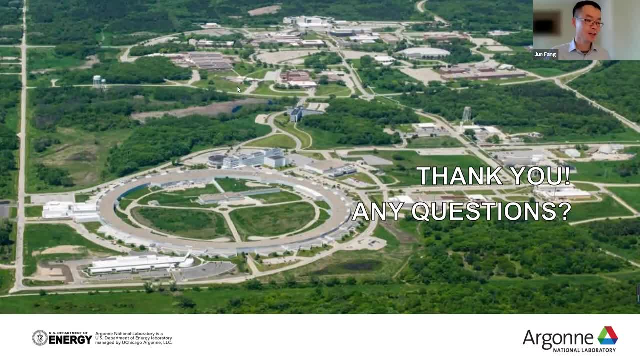 simulation? Yeah, So we have. There's a, A, The, The System. That's right For Baroni Method. So where We have a dedicated Program that calculate the Position of the pebbles. 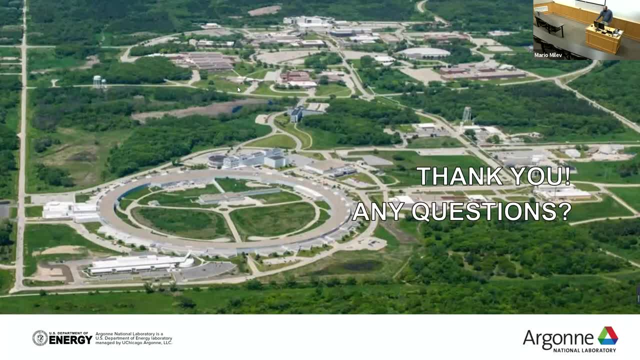 For randomly packed pebble? Yes, Okay. Next question: Is Our momentum source terms Added in all the cells Or of the spacer grids? So the momentum sources are only added in the locations where we expect the spacer grid and mixing lens to be. 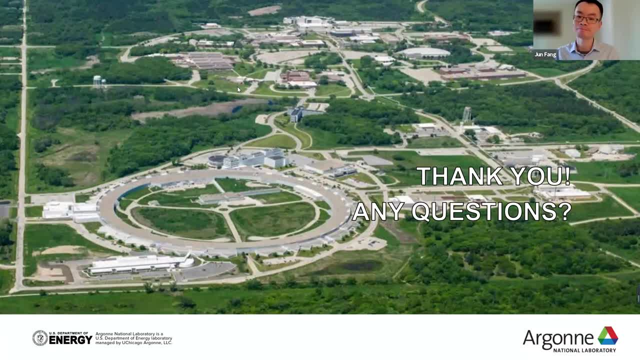 So it's not applied to all the cells. OK, and in doing that, do you use a structured mesh for the LES study with spacer grids? No, it's unstructured. So for the LES reference simulations we did it with the unstructured mesh. 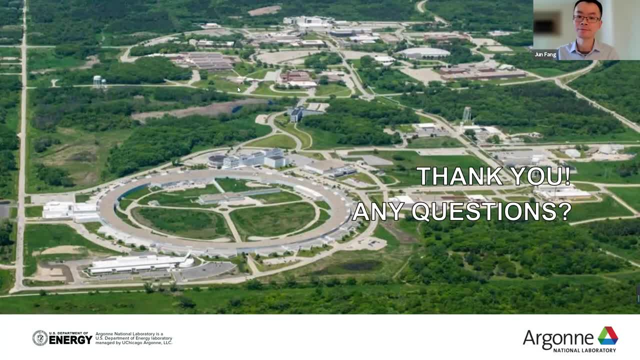 But for the RANS simulation it's a structured mesh. I hope it clarifies it And if there's any follow-on questions for any of the questions that are being asked in the chat, please feel free to post them if you'd like, or raise your hand. 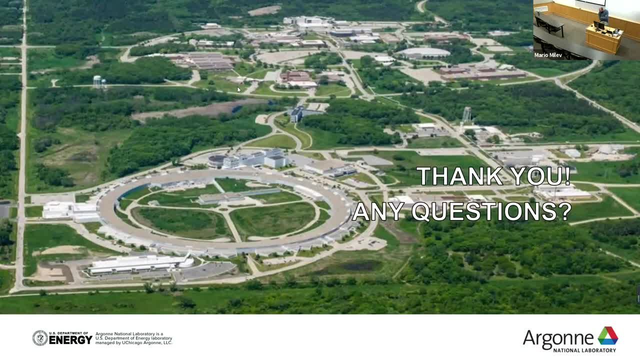 One last question I see here on the chat is: is there any best practice to extract most useful data and information from the full-core simulations? That's a good question, So I think so here the so we let me think. 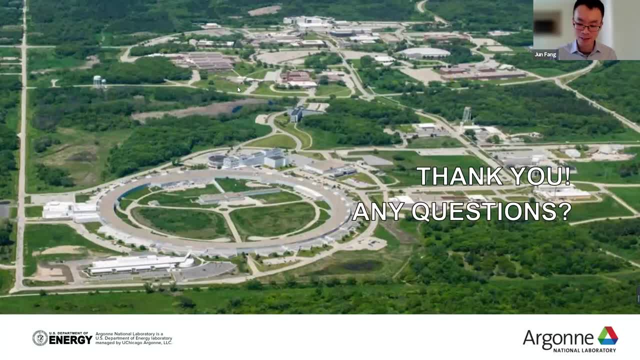 How can I put this? So for right now, we only extract the range of the design parameters, such as the range of temperatures in the fuel, in the fuel in the solid region and the temperature in the cooler region. I think it would be very useful to monitor. 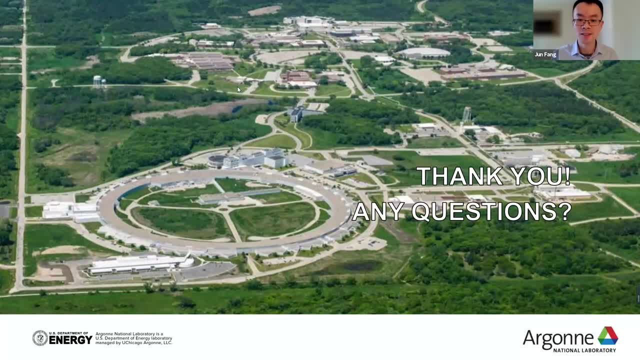 the ranges of these values from the simulations. And Yeah, I'm not. I think that's what we have been doing for now. Thank you very much. If I may one question? Sure, Yeah, take the ball down, Yeah. 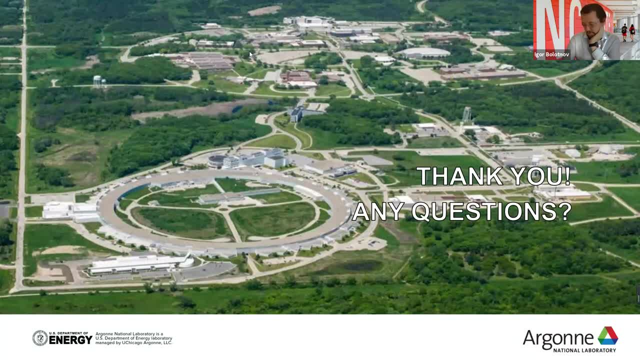 So Jun, very interesting, very good presentation. Thank you very much. So for the Reynolds number, when you deal with RANS, I mean we all know what, when we deal with DNS or LAS, the computational cost implications, Right. 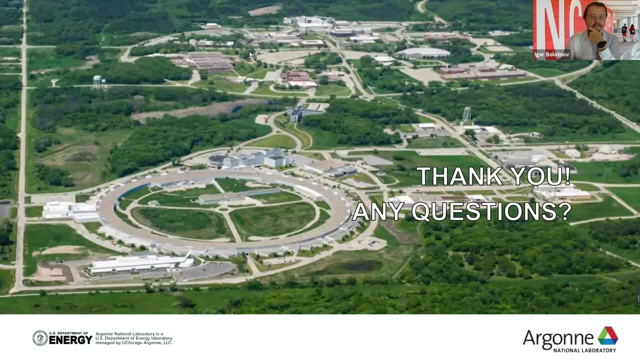 So with RANS shouldn't it be in? I mean, you have to resolve the boundary layers somewhat, but the bulk mesh is not that. I mean. is it, do you know, like the exponent computational cost growth? is it the same or is it smaller for RANS? 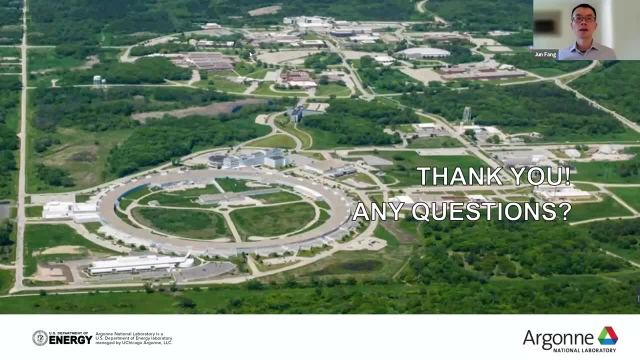 as you increase the Reynolds number. So, as I mentioned the specific RANS models we have, it's the more resolved RANS models OK, Which means we still have a fine resolution near the wall And the rule of thumb there is to keep the first layer of mesh. 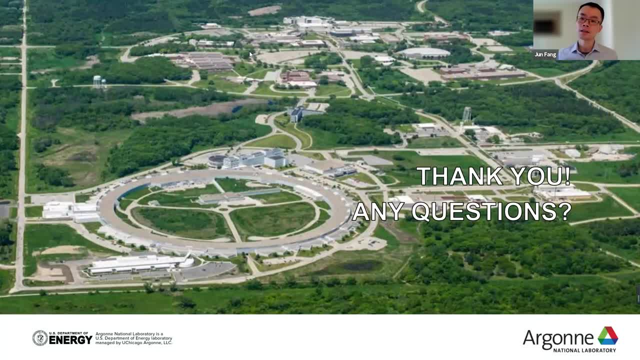 of the wall to be under the Y plus of one, And in the bulk region it's much more tolerant And I think the overall like the ratio, the mesh size increase ratio. in terms of the Reynolds number it's lower than DNS, for sure. 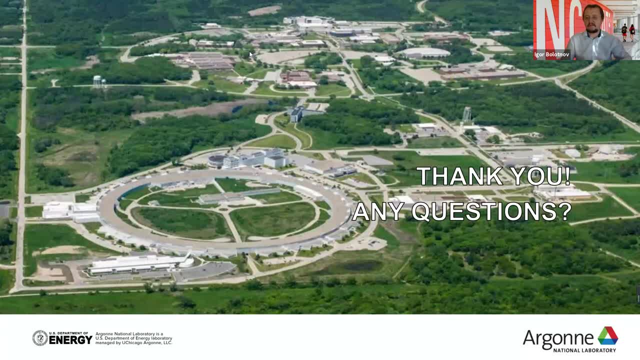 Yeah, You can keep. the bulk is sort of coarse, I mean it's only flatter where it's boundary layers. Yeah, Right, And another follow-up question: That's the reason we're developing this wall functions, capabilities, to kind of overcome this limitation of more resolved. 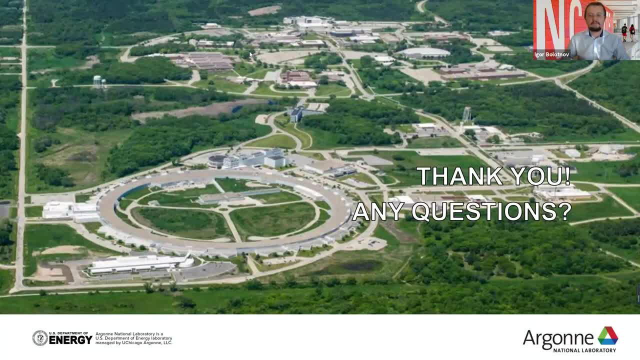 RANS. So like better high Reynolds number type of Right right, right right. So that's kind of the motivation of our wall function. Yeah, OK, And the follow-up on momentum sources, do you have to? and I don't know. 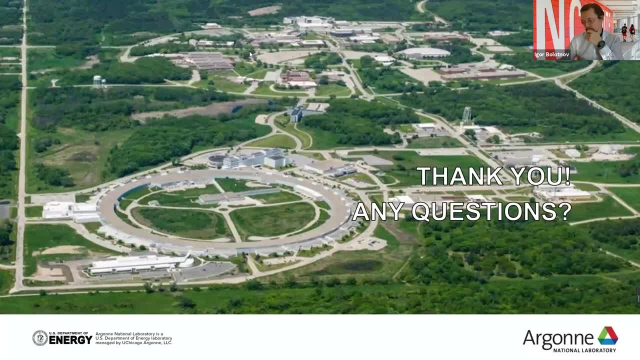 maybe I missed something, but as you work at different Reynolds numbers, do you have to completely redesign the momentum sources or remodel them, or remodel this kind of universal? Yeah, It's not universal yet. We have to do some recalibration if we want to. 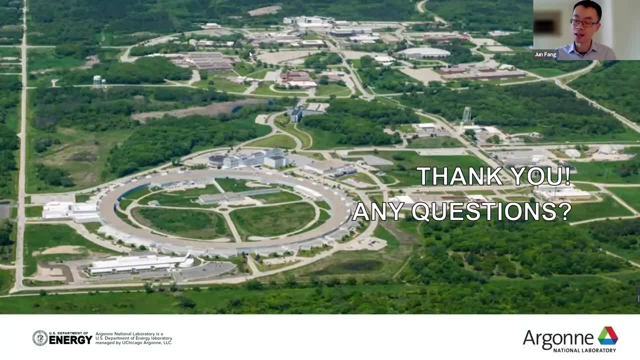 Actually I didn't mention it. Yeah, Yeah, Yeah. So when we did our presentation we did the LES reference simulations for multiple Reynolds numbers from the basic like 10k, no, yeah, 10k to 80,000.. 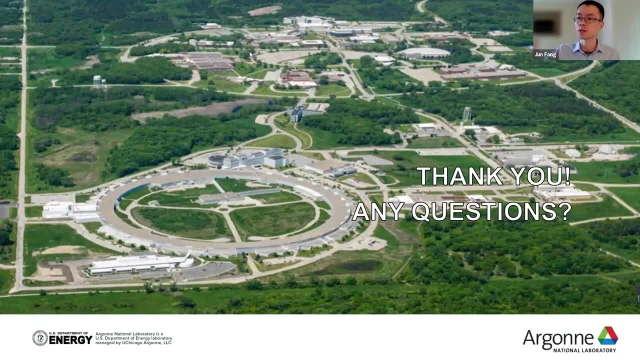 So, if we need, we can do some interpolation between the Reynolds numbers. Thank you, Mm-hmm. OK, Last chance for questions from the One from one of our- one of our in-person participants, So go ahead Yeah. 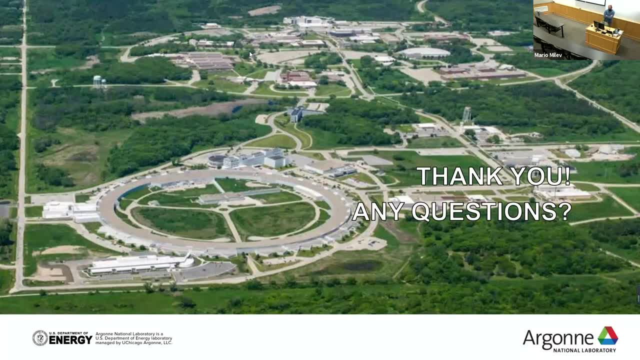 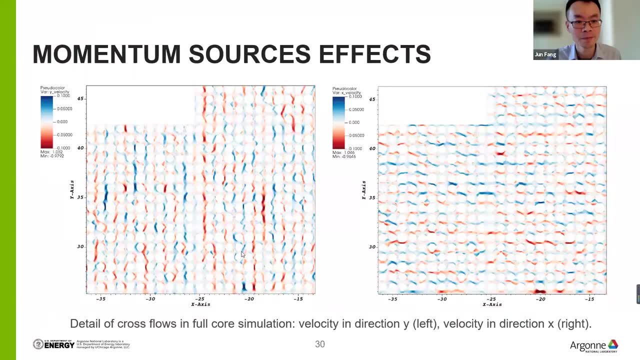 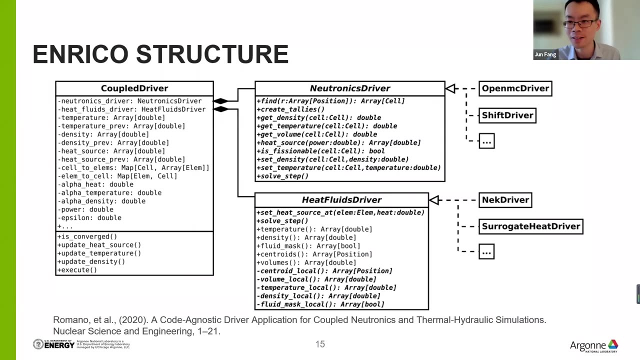 So you showed on one of the slides a reference for people who are interested in the multi-physics coupling between the electronics and thermal hydraulics. Do you have that slide so I can get that This one or the one before This one? yeah,